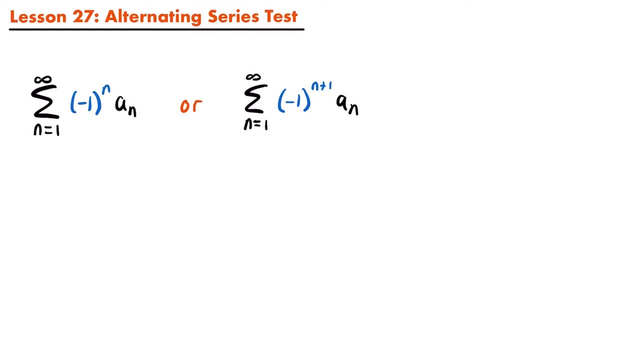 So, if you remember, if we have a sequence, a sub n that is equal to negative one to the power of n, the terms will look like this: When n is equal to one, we have negative one to the first power, and so that's negative one. Then the next term is when n is equal to two, and so negative one. 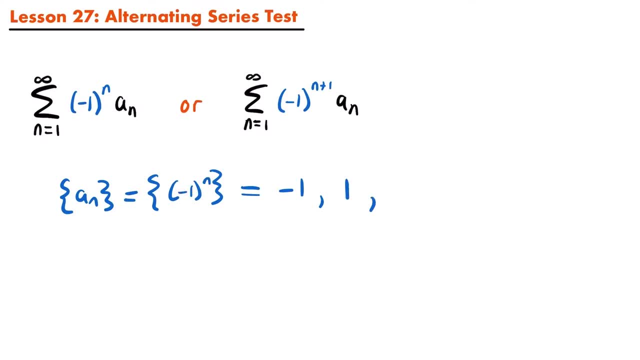 squared, is positive one, and these terms will continue to alternate between negative one and positive one from there on out. So we're going to look at some series that have both positive and negative terms. When this power of n is even, the term will be positive one, and when n is odd, 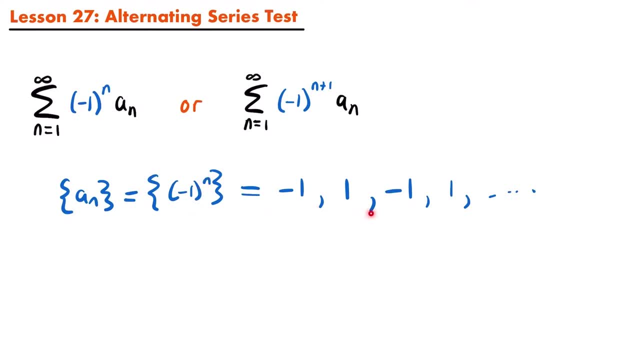 the term will be negative one. And so we have this sequence of alternating terms between negative one and positive one. And then, just as a comparison, if a sub n was equal to negative one, to the power of n plus one, that would just change the order of our alternating terms Instead of starting with. 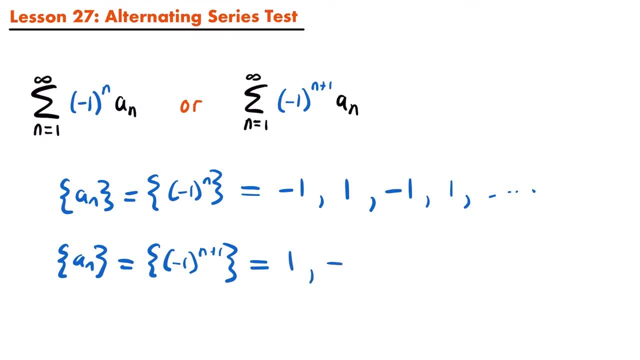 negative one, we would start with positive one, and then we'd go to negative one, Then we'd go to negative one, then positive one, and so on. Right, Because of this plus one. now, when n is an odd number, 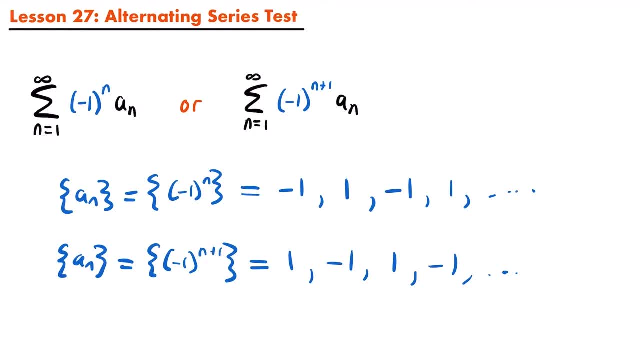 it's going to become an even number because we're adding one to it And so that will output positive one. and when n is an even number, adding one to it makes it an odd number, and so that outputs a negative value. Okay, So that's just a little bit of a refresher on negative one to the power. 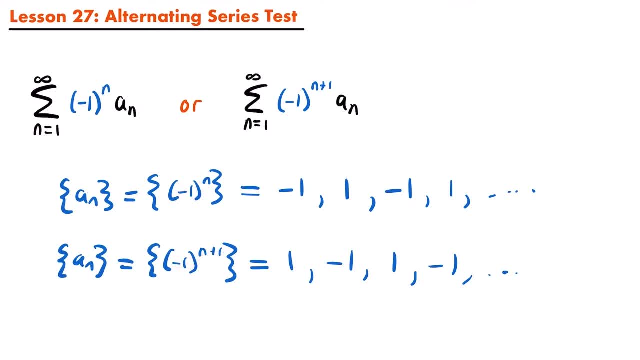 of n or negative one to the power of n plus one. And because these two sequences alternate in their signs, multiplying either of those by another sequence, a sub n, is going to result in a series that has alternating terms, right? So for example, let's say we had the series: the sum from n equals one to infinity of negative. 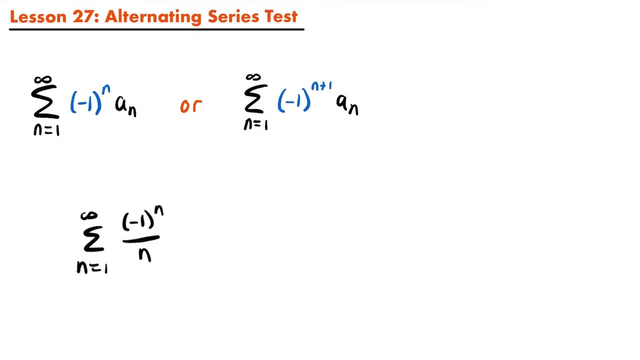 one to the power of n divided by n. What would the terms of this series look like? Well, if we wrote them out, when n equals one, we have negative one to the first power, which is negative one divided by one. So our first term is negative one. 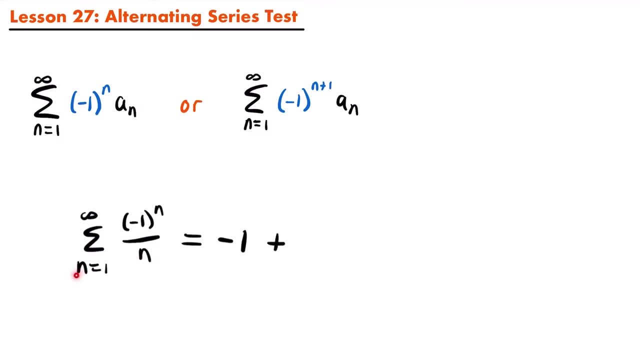 Then we will add that to the second term where n equals two. So now we'll have negative one squared, which is positive, one divided by two, So now we have one half. Then our next term, when n equals three, we'll have negative one cubed, which is negative. 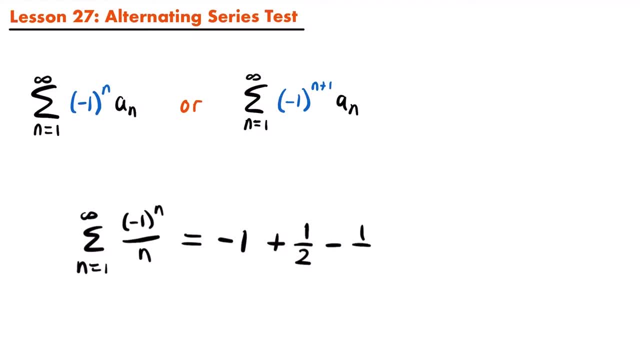 one divided by three. So now we are subtracting one third, okay, And then one more. When n equals four, we have negative one One to the fourth power, which is positive one divided by four, And so we add one fourth, all right. 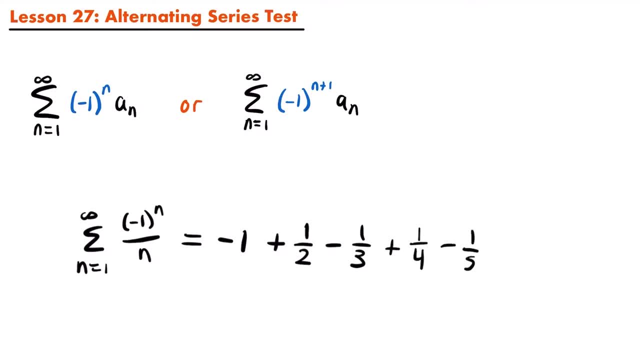 And so then, if we were to continue on, we would have negative one fifth plus one sixth minus one seventh, and so on. all right, And so you can see that, because of this negative one to the power of n, the sign of our terms, 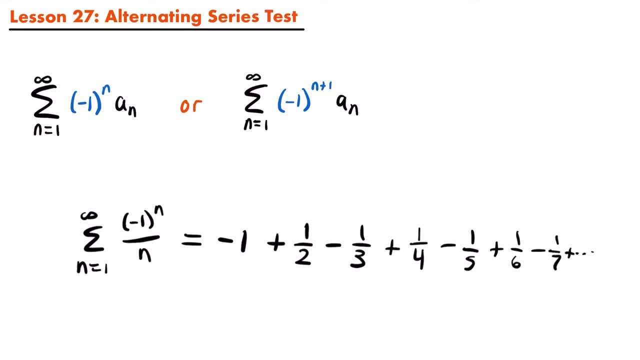 alternates between being positive and being negative, And so, in order to determine if an alternating series like this series right here can converges or diverges, we can use a special test, And that test is what we call the alternating series test. 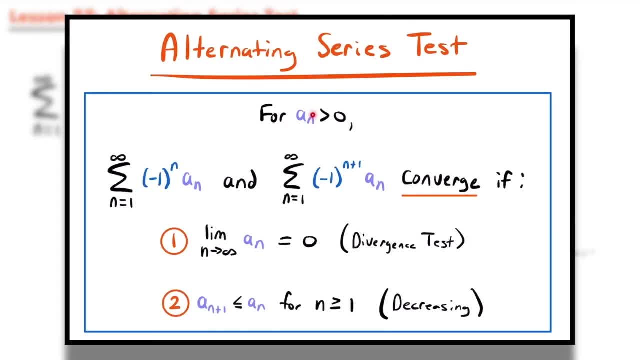 And here's what the alternating series test says For a sequence: a sub n greater than zero, meaning that that sequence is a positive sequence. these two forms of an alternating series where we have negative one to the power of n times that sequence, a sub n, or negative one to the power of n plus one times that. 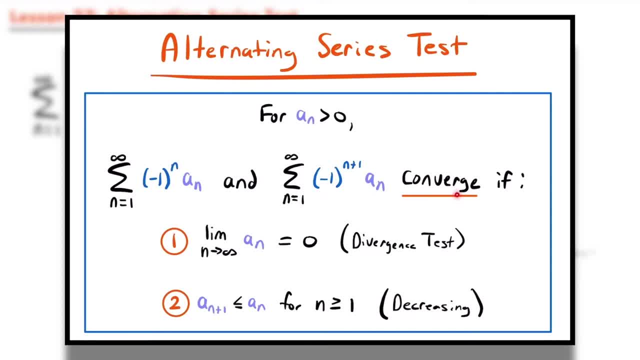 sequence. Those two alternating sequences will converge If these two requirements are met. The first one is that the limit as n approaches infinity of our sequence needs to be equal to zero. Essentially, what we're doing here is using the divergence test. Remember that we would take the limit as n approaches infinity of the sequence for 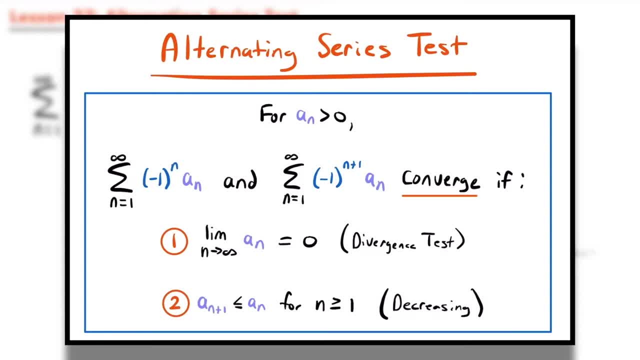 our series, And if that wasn't equal to zero, then we could conclude that the series diverges. And so what we're saying here, with this first requirement, is that the divergence test will fail right. The limit, as n approaches infinity, of a sub n needs to be equal to zero, which means that 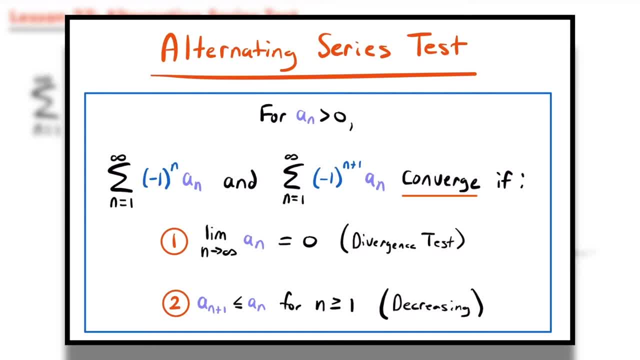 our series could converge or it could still diverge, but we don't know, based on the divergence test. All right, so that's the first requirement that needs to be met. The limit, as n approaches infinity of that sequence needs to be equal to zero. 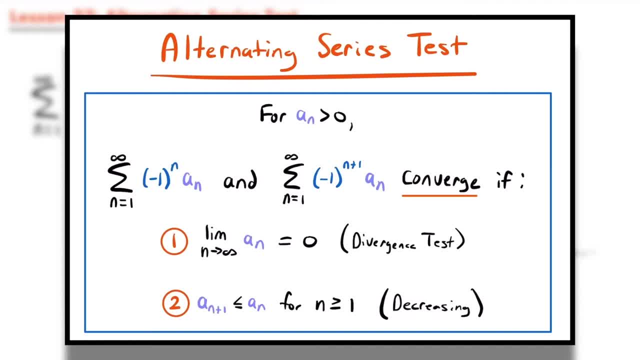 And then the second requirement is that our sequence needs to be a decreasing sequence. The next term of the sequence, a sub n plus one, needs to be less than or equal to the previous term, a sub n. And that needs to be true for n greater than or equal to one or all values of n for the. 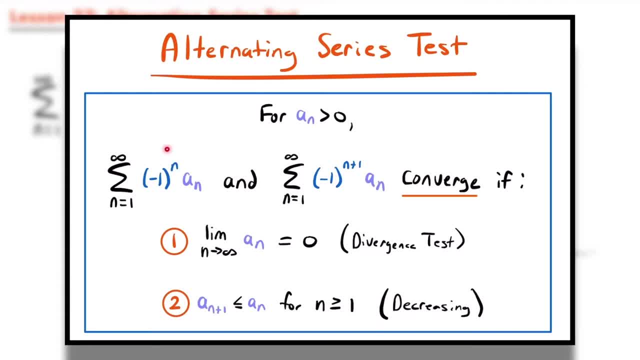 sequence. Okay. so if we can show for an alternating series that the sequence a, sub n fails the divergence test and is a decreasing sequence, we can conclude that our alternating series converges, All right. And so, before we look at some example problems of using the alternating series, test for some. 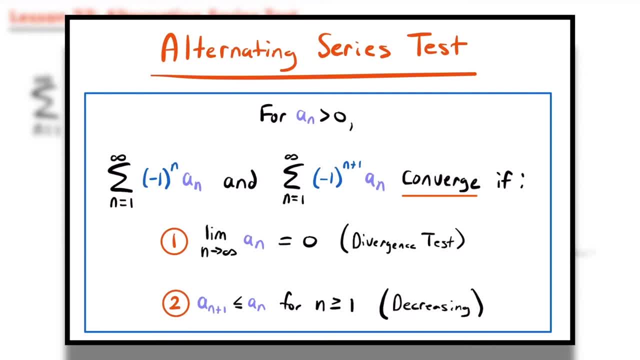 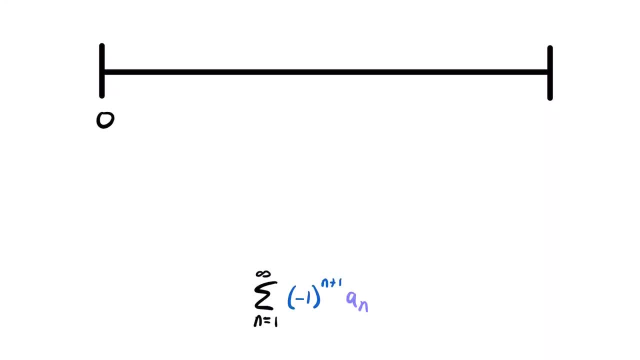 alternating series. I want to quick show you a nice visual that will maybe help you understand why the alternating series test works. Okay, so here I have a number line, And what this number line is going to represent is the value of the sum of an alternating 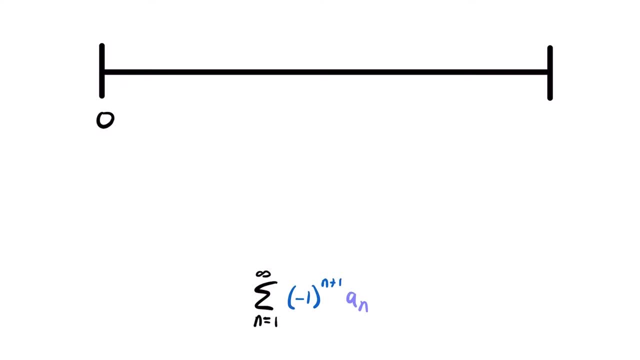 series. Now we're specifically going to look at this form of an alternating series, where the first term would be positive. But note that this demonstration would also work for the other form of an alternating series as well. But I'm just going to focus on this form right here. 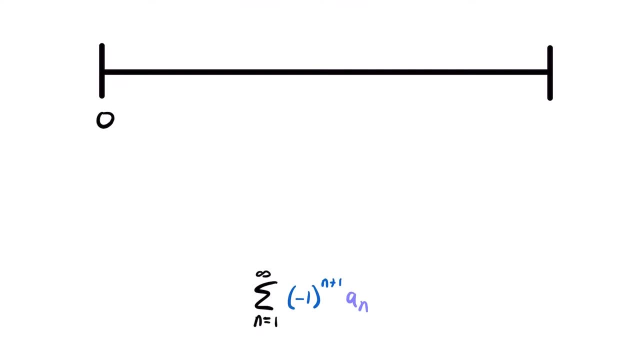 Where that first term will be positive, And what we're going to do is assume that this alternating series converges, which means that this sequence- right here, a sub n, would be a decreasing sequence, Meaning that if we ignore the sign produced by this part of the series, each subsequent 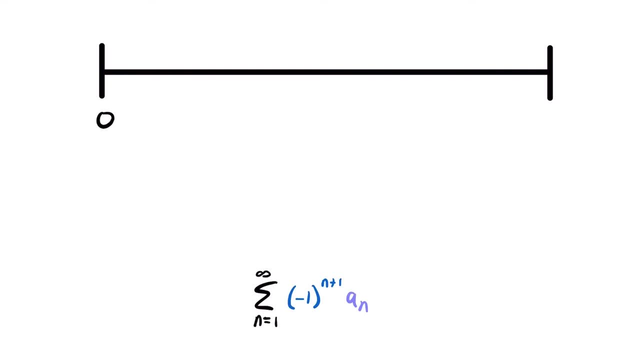 term of our sequence would be smaller than the previous term. Okay, so keeping that in mind, let's say we were to calculate the first partial sum for this series, right? All that would? All that would involve is looking at the first term of the series, okay. 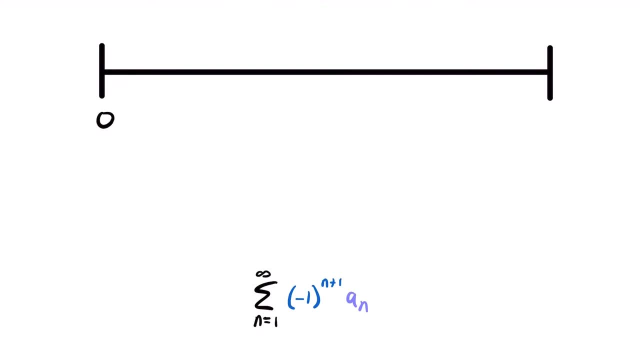 So if the sum of our series starts at zero because we haven't added anything yet, but then we add the first term of the series, that will take us to a value that we are going to label with s sub one, the first partial sum. okay, 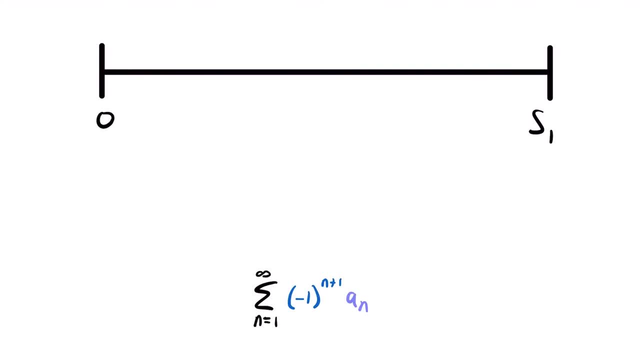 And so that first term is positive for this series. but then if we add the second term to get the second partial sum, that second term is negative, And so the second partial sum will be smaller than the first partial sum. We're going to move backwards a little bit in the value of the sum, right? 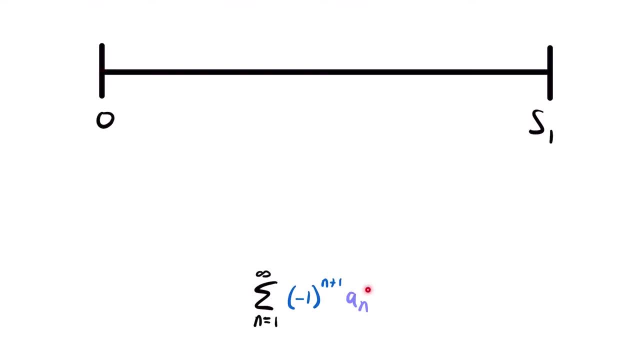 But we're not going to move all the way back to zero because the terms of our sequence are decreasing, And so we could say that right about here would be the value of the second partial sum. Now, if we add the third term of our series, that term is going to be positive again. but 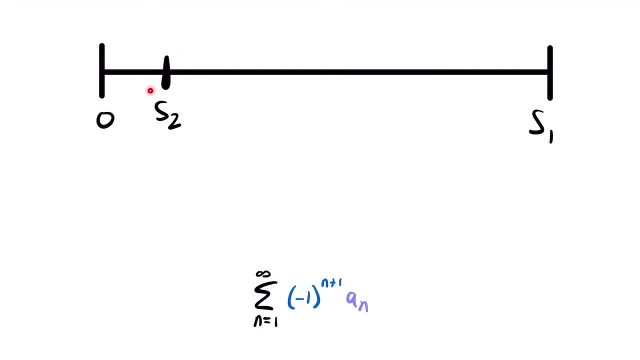 we're going to be adding a smaller amount than we subtracted to get s sub two, So the third partial sum would maybe be right about here, And so we could label that with s sub three. And then if we added the fourth term of the alternating series, that value will be negative. 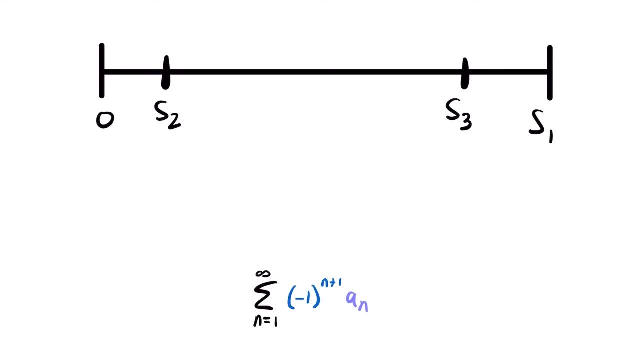 again, We're alternating between positive and negative, And so the value of our sum is going to get smaller again. We're going to move from this value of s sub three to a smaller value, but it will still be bigger than s sub two, because each term is still getting smaller, regardless of the 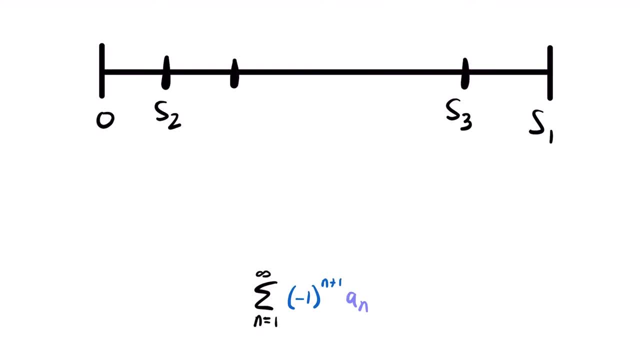 negative sign or not. And so the fourth partial sum we could say is right about here. Okay, Right about here. And then, if we were to look at the fifth term, we would once again add a term. it would be positive again. 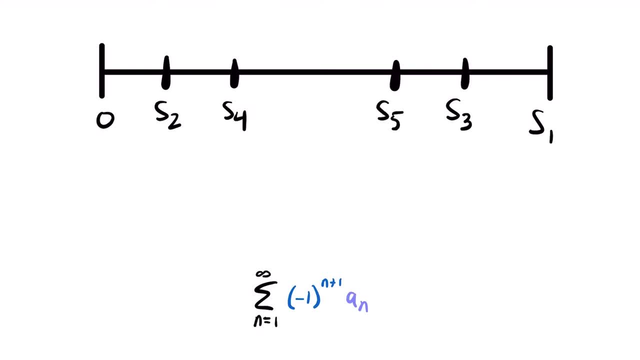 So we could say that this is s sub five, And if we added another term to get s sub six or the sixth partial sum, we would now be subtracting another term And so this could be s sub six. And, as you can see, as we continue to add more and more terms of a converging alternating 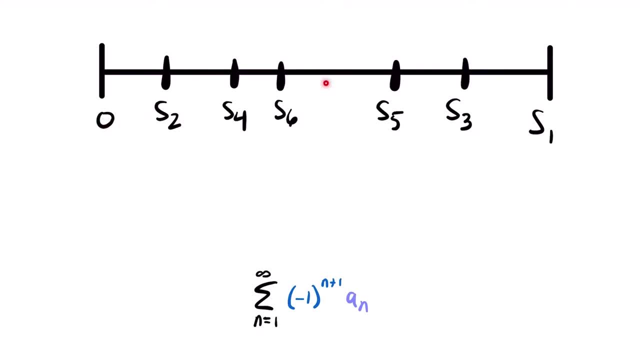 series. the sum of the series is slowly converging to a value Right. So if we were to calculate a couple more partial sums, s sub seven would be right here, And then we could do one more with s sub eight. that would be right here. 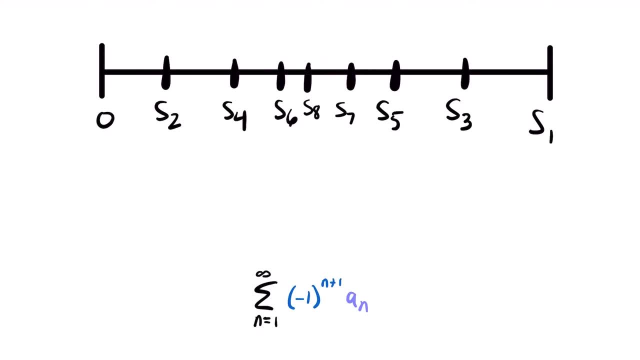 And you could see that we are getting closer to some value between zero and our original partial sum. Okay, So, because each term of the sequence is getting smaller and the signs of those terms are alternating, we have this back and forth motion that is occurring with the partial sums that 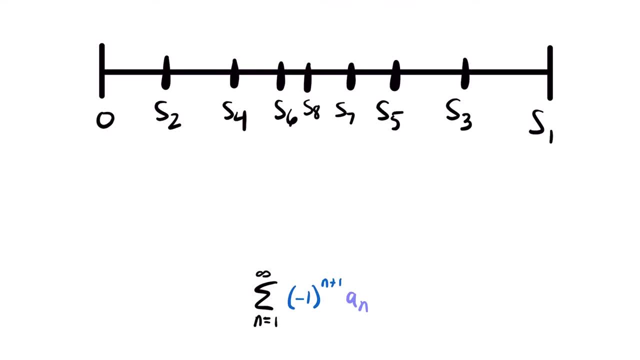 will eventually converge to some value. To some value: that is the sum of the alternating series. Okay, So that's why it's important for an alternating series to have a sequence that is decreasing in order for it to converge. Okay, And so hopefully, this was a helpful visual for understanding why the alternating series. 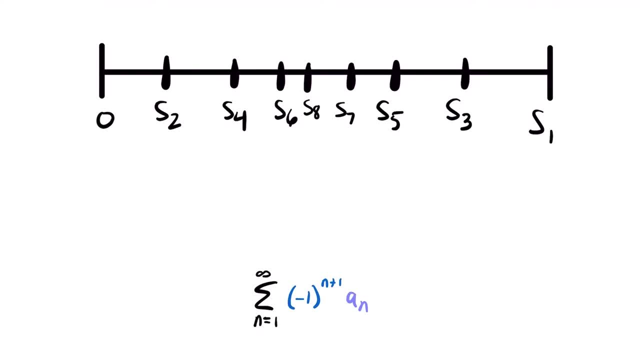 test works All right, And so with that, let's look at some examples of using the alternating series test to determine the convergence or divergence of an alternating series. Okay, so here's our first example. We have this series: the sum from n equals one to infinity of negative, one to the power. 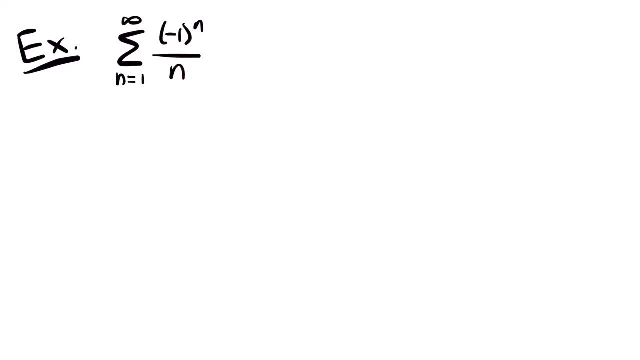 of n divided by n. All right, And now it's pretty easy to identify an alternating series, because if you see negative one raised to a power of n, or n plus one or n minus one or anything like that, you immediately know that you have an alternating series. 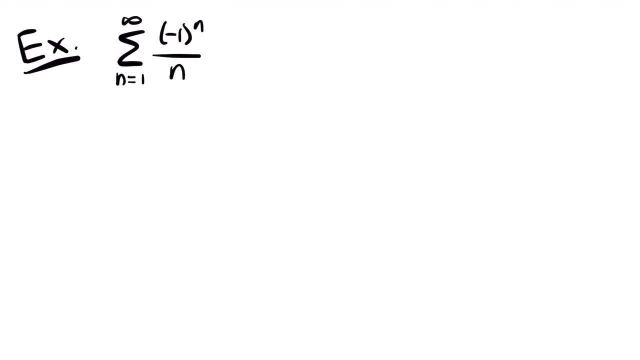 And so, in order to determine if it converges or not, you're going to want to use the alternating series test. And so, for this series, can you identify what the sequence a sub n would be? Well, if we rewrote this a little bit, this is equal to the sum from n equals one to infinity. 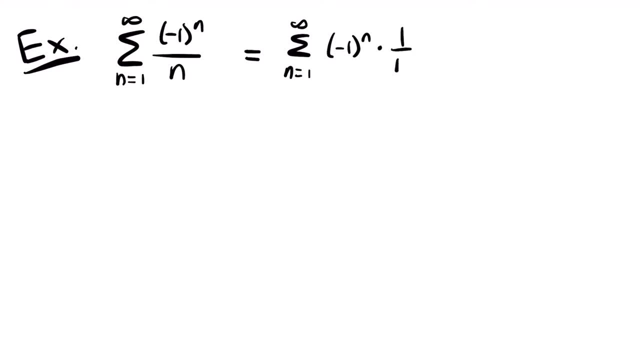 of negative one to the power of n times one divided by n. Right, We just had negative one to the power of n divided by n, So we could pull that out And now you can see the two parts of our series. We have the negative one to the power of n, which makes this series an alternating series. 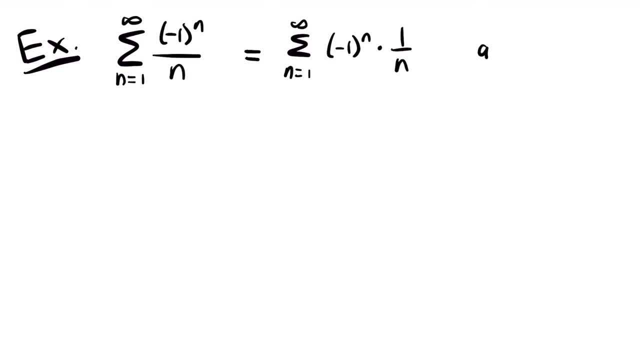 Okay, This is the sequence. a sub n. All right, So a sub n is equal to one divided by n. Okay, And so just a quick side note, without this negative one to the power of n. hopefully you are familiar with that series. that would be left over. 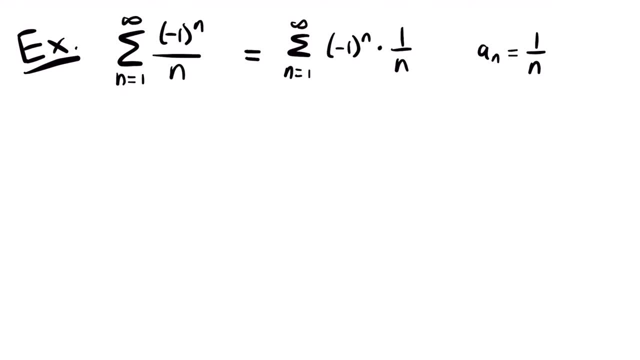 Without this part, we would just have the sum from n equals one to infinity of one divided by n. That is the harmonic series, which is a p-series where p is equal to one, And so we actually call this series, right here, where you have that harmonic series. 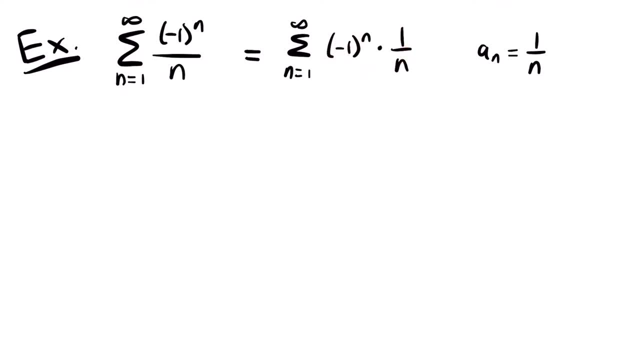 but it's alternating the alternating harmonic series. Okay, But putting that aside, we now want to use the alternating series test to determine if this series converges or diverges, And so the first thing we need to do, our first step, is to take the limit as n approaches. 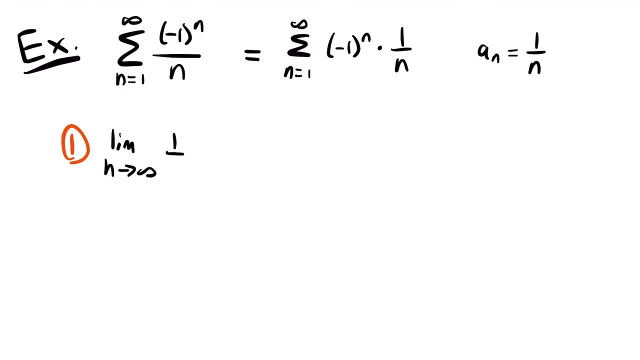 infinity of our sequence, a sub n, which is one divided by n. All right, And so what happens to one divided by n as n approaches infinity? Well, when you have one divided by n, where n approaches infinity, you have one divided. 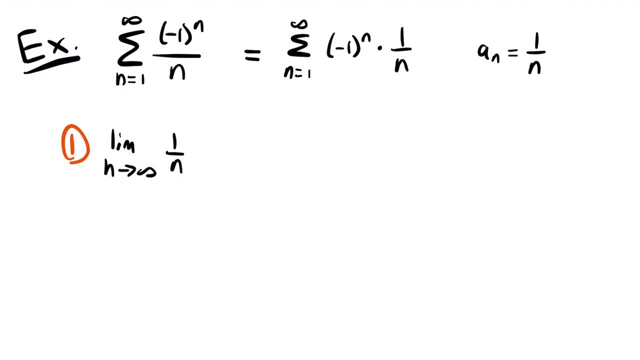 by n. When n approaches infinity and that denominator is getting larger and larger, a fixed value of one divided by that increasing denominator will always be equal to zero. All right, So the limit as n approaches infinity of one divided by n is equal to zero. 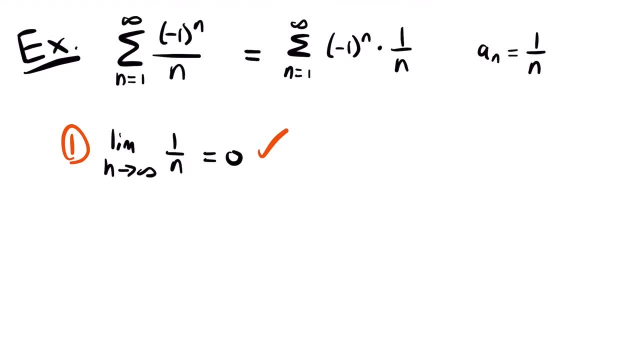 And so our first requirement is met. We have checked to make sure that the limit, as n approaches infinity, of our sequence is zero, And now we can check our second requirement. We need to show that our sequence is dn, And now there's two different ways that you could do that. 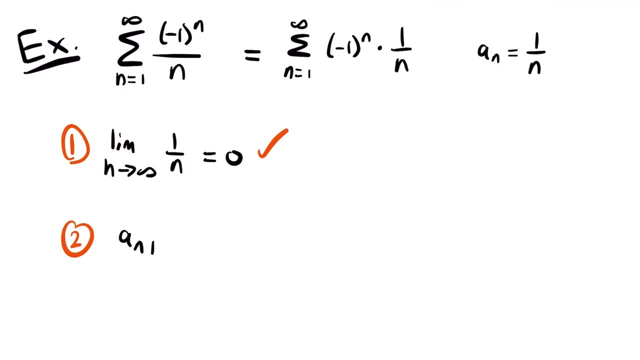 You could do a term by term comparison by looking at the term a sub n plus one and showing that it is less than or equal to a sub n, And that would need to be true for all values of n, meaning values of n from one to infinity. 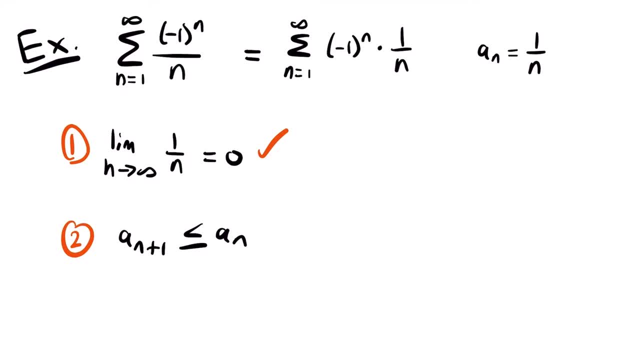 Or you could look at the corresponding function to the sequence. So you could look at: f of x is equal to one divided by x. We just replaced n with x and made it a function And you could take the first derivative of this function. 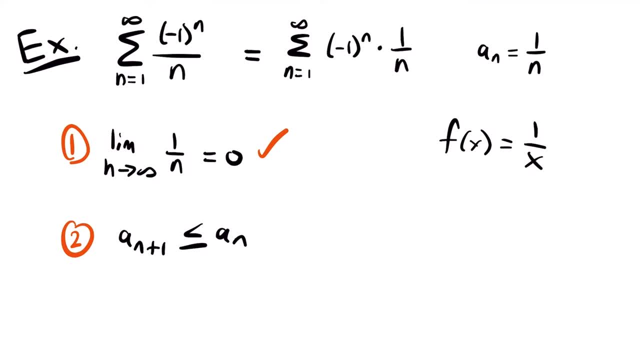 And if that derivative is negative for all values of x, from one to infinity, then you could also say that your sequence is decreasing. All right, But in this case I'm going to use this first method. I'm just going to look at the term a sub n plus one and a sub n and conclude whether. 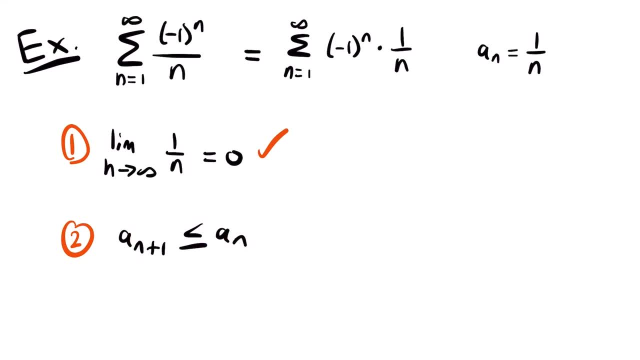 that term is less than or equal to a sub n. All right, So in this case a sub n plus one will be one divided by n plus one, since we replace n with n plus one And then we just have one divided by n. 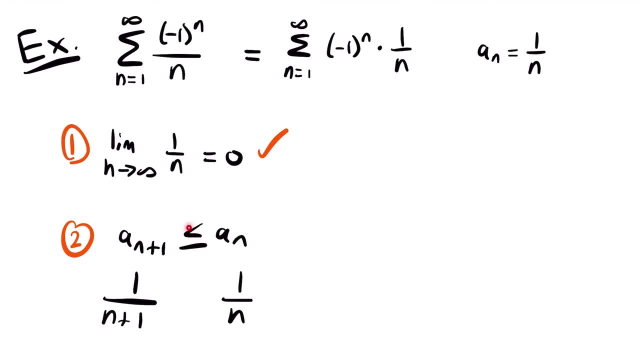 For a sub n. Now is this term less than or equal to this term? Well, if you look at the denominators, we have n plus one and n, And so this denominator will be larger than this denominator. And when you increase the denominator for a fraction, the value of that fraction gets. 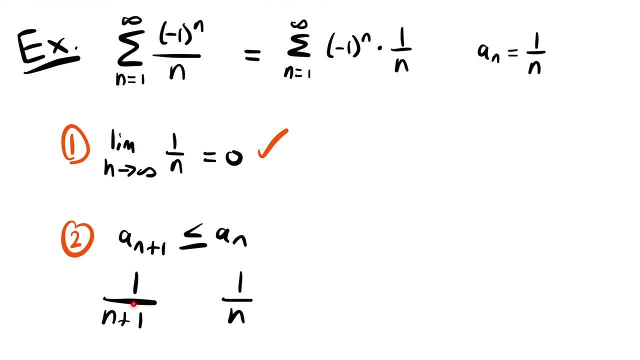 smaller, And so we would say that one divided by n plus one must be smaller than one divided by n, since the denominator is larger, And so So this statement is true- It is less than or equal to one divided by n, And so now we have shown that this series meets both of these requirements for the alternating. 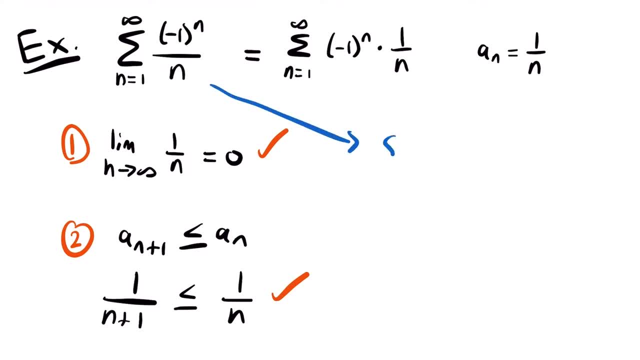 series test And so we can conclude that our series converges. All right, And that's really all there is to the alternating series test. You take the limit of your sequence as n approaches infinity, show that it is zero and then show 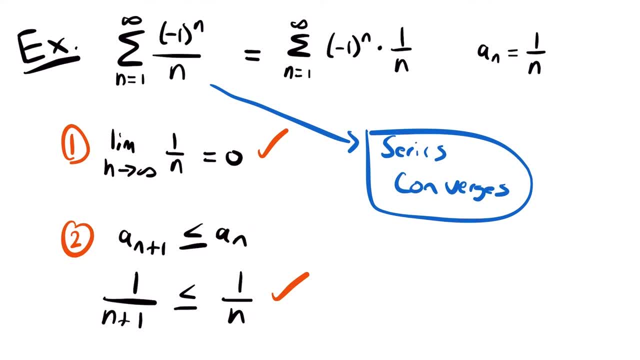 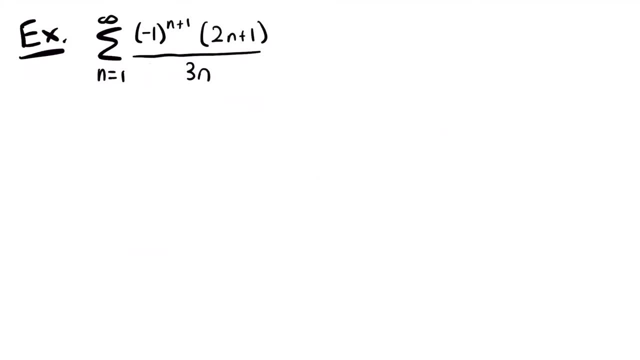 that your sequence is a decreasing sequence, And if those are both true, then you know for a fact that your alternating series converges. All right, Let's look at another example. Okay, So here's our next series. We have the sum from n equals one to infinity of negative, one to the power of n plus one. 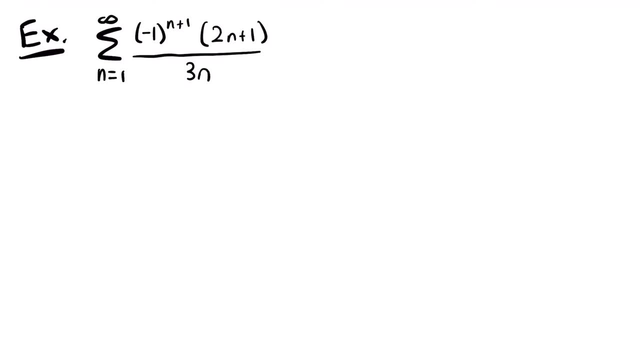 times two n plus one, divided by three n. All right, And so right away we can see that this is an alternating series because of this negative one to the power of n plus one. That is a dead giveaway that this series is an alternating series. 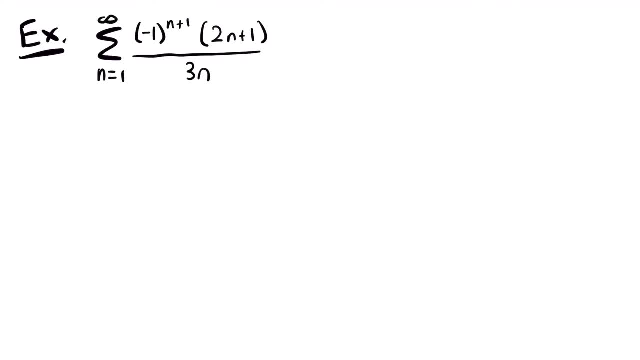 All right, Let's look at another example. So here's our next series, And so we know that, in order to determine if it converges or diverges, we need to use the alternating series test, And so, in order to do that, we need to identify what our sequence is. 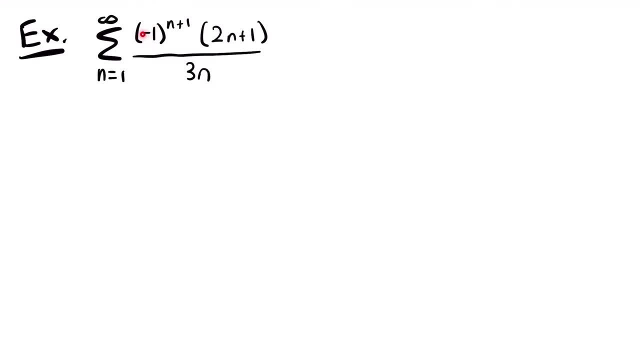 And so the easiest way to do that is just to remove this negative one to the power of n plus one from the series, And then you'll have your sequence right. So a sub n will be equal to two n plus one divided by three n. 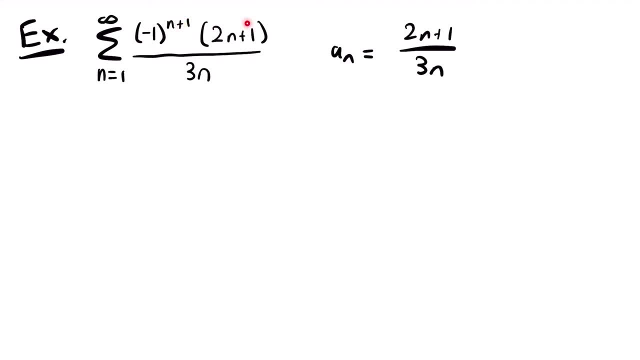 We just removed negative one to the power of n plus one, And we're left with this quantity divided by three n, And so that is our sequence. Okay, And so now let's check our two requirements. Let's first check to see if the limit as n approaches infinity of our sequence is equal. 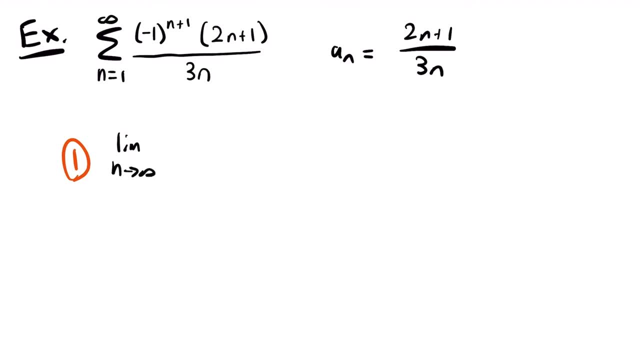 to zero, And so we'll take the limit, as n approaches infinity, of two n plus one divided by three n. Okay, And so now, how can we evaluate this limit? Well, there's a couple of different ways that you could do it. 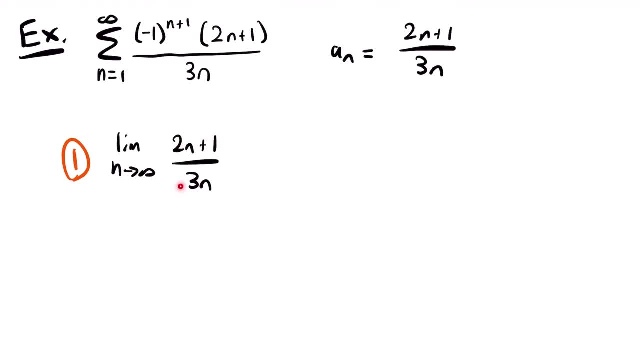 You could use L'Hopital's rule if you wanted to, because the numerator and denominator, as n approaches infinity, would both be infinity right, As n gets larger in the numerator. two times an increasing value plus one is just going to keep getting larger and larger. 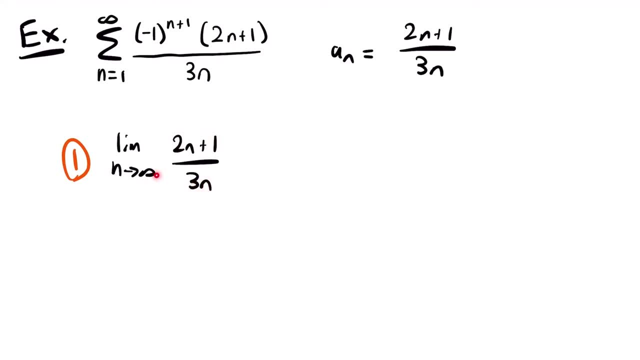 And so that is infinity. And three times n, where n is approaching infinity, is also increasing towards infinity, And so this is in an indeterminate form that is compatible with L'Hopital's rule. So you could take the derivative of the numerator and denominator and evaluate from there. 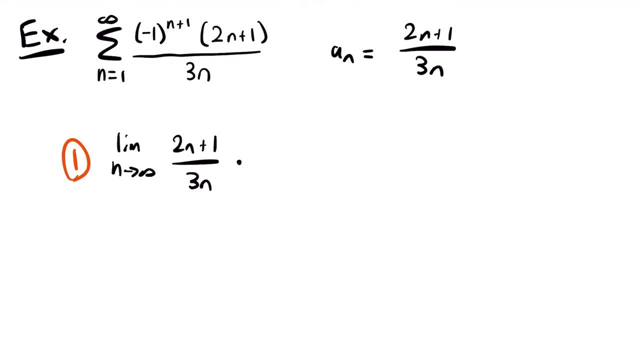 Or you could use the method I'm going to use here, Which is just to multiply by a form of one of one divided by n to the highest power found in the numerator or denominator. In this case, that's just n to the first power. 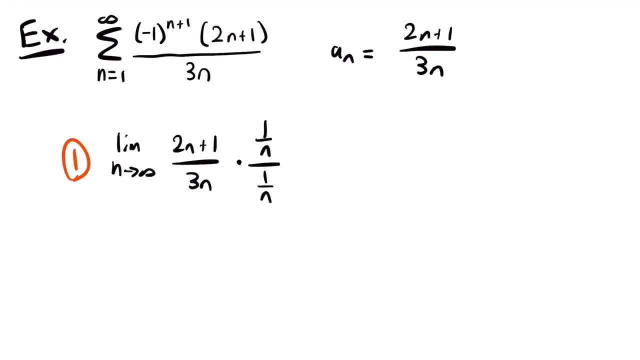 So multiply by one divided by n divided by one divided by n, And doing that will give us the limit, as n approaches infinity, of two plus one divided by n divided by three. right Two n times one divided by n. those n's cancel out and leave us with two and one times one. 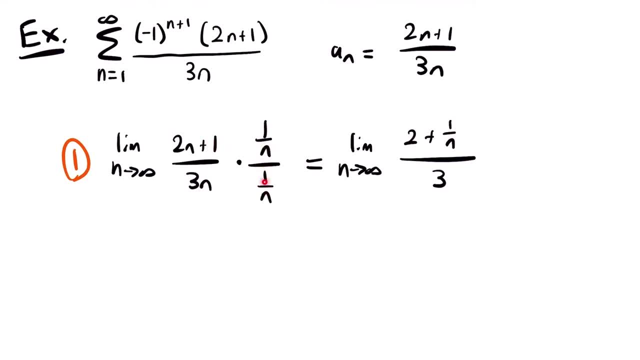 divided by n, And then three n times one divided by n. those n's cancel out and leave us with three. Now, the limit, as n approaches infinity of one divided by n, is zero, And so this is equal to two plus zero divided by three, which is equal to two thirds. 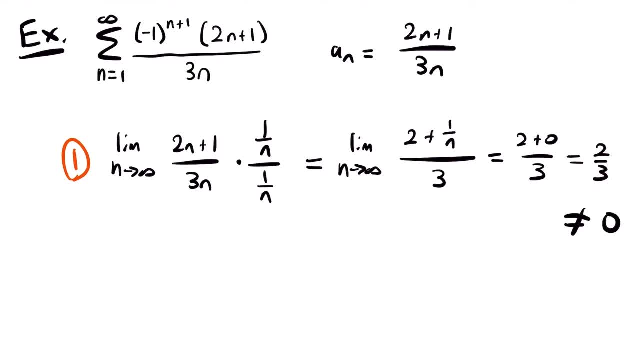 And two thirds is not equal to zero, And so our first requirement for the alternating series test is not met. okay, And so because of that, we don't even need to check the second requirement. Instead, what we have shown here is that, via the divergence test, that this series diverges. 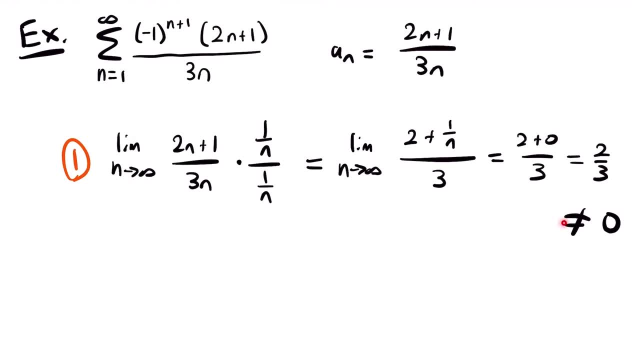 The limit as n approaches infinity of our sequence is equal to a value that is not zero, and so our series must diverge, okay? So since we found that the limit as n approaches infinity of our sequence is not zero, we can make the conclusion that this series diverges okay. 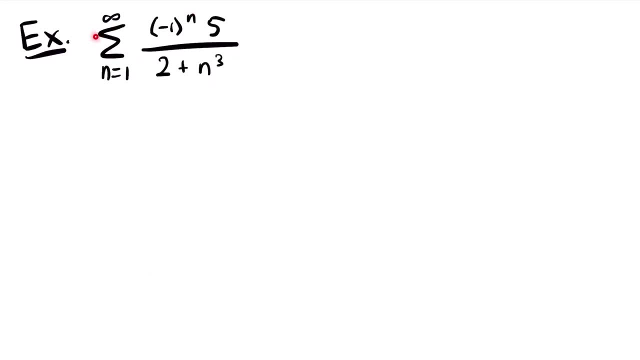 Let's look at another example. All right, So for our next example we have the sum from n equals one to infinity of negative, one to the power of n times five divided by two, plus n to the third power. All right, So once again we immediately can identify this as an alternating series because we have 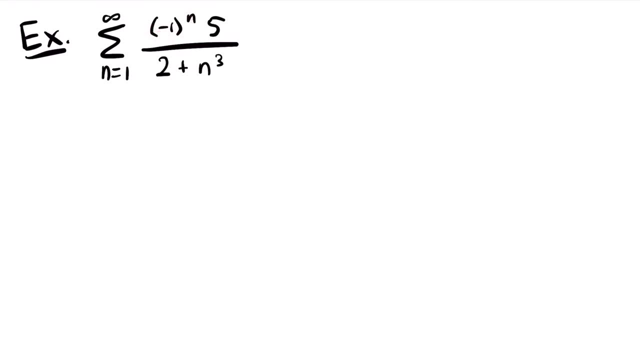 negative one to the power of n. So we know that we can use the alternating series test to determine the convergence or divergence of this series, And so the first step of the alternating series test is to identify our sequence. Okay, So what is n equal to? 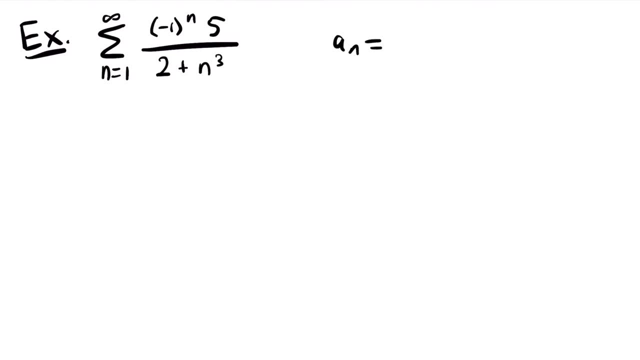 Well, all we have to do is block out this negative one to the power of n and then just rewrite everything else. So we have five divided by two plus n to the third power. Okay, And so now we will look at the first requirement for the alternating series test. 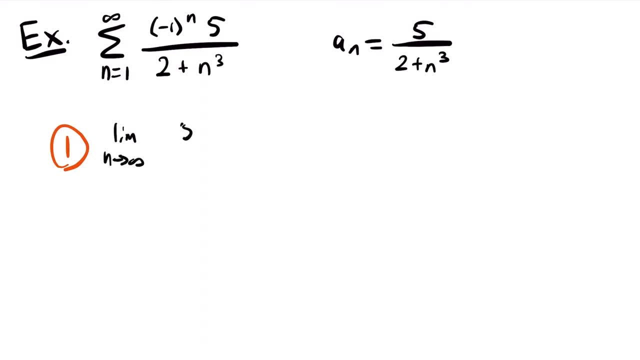 We will take the limit, as n approaches infinity, of five divided by two plus n cubed. And so what happens to this expression? as n approaches infinity, Well, we can calculate the convergence of n as n approaches infinity. as n approaches infinity approaches infinity, Well, we only have an n in the denominator, and as that n approaches infinity. 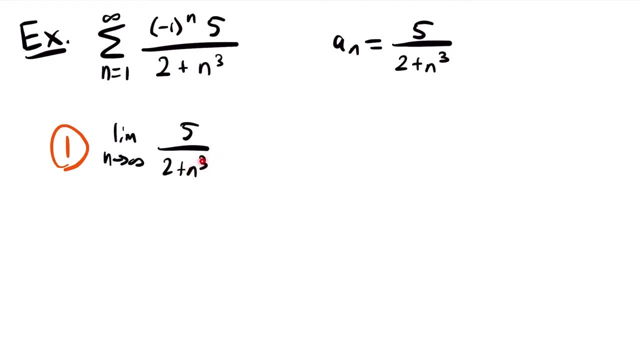 meaning it is getting larger. we are cubing that value and then adding it to 2.. So this denominator is going to increasingly get larger and larger as n approaches infinity. And so we have a fixed value of 5 divided by an increasing denominator, which is always going to approach 0 as n approaches. 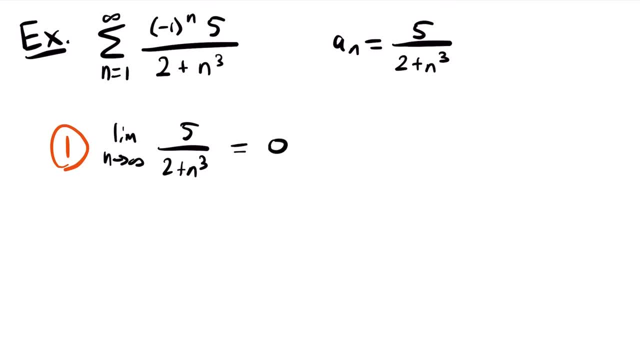 infinity, And so this is equal to 0.. So our first requirement is met. Alright. now what about the second requirement? Let's check to see if this sequence is a decreasing sequence. What we want to know is: is it true that a sub n plus 1 is less than or equal to a sub n? Is the next term of the? 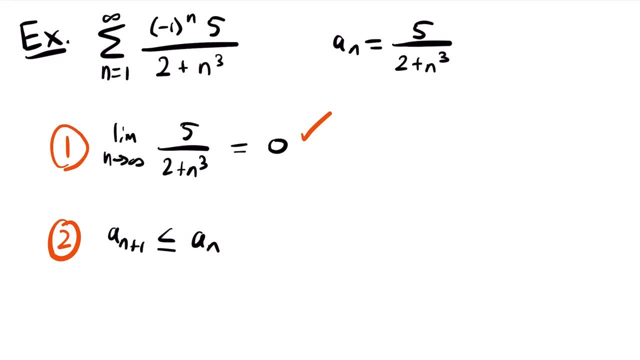 sequence smaller than the previous term. And so if we look at a sub n plus 1, that will be 5 divided by 2 plus n plus 1 cubed, And then a sub n is just 5 divided by 2 plus n cubed. Now if we compare these two fractions, 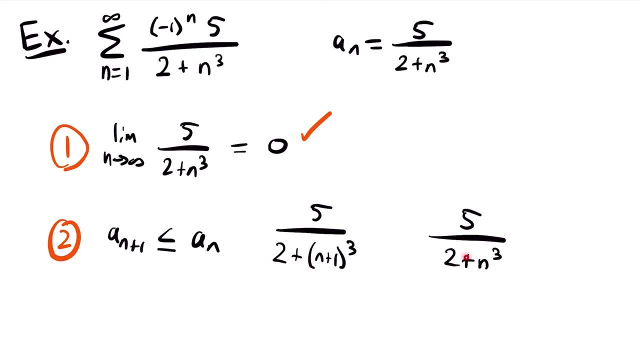 note that this denominator will be larger than this denominator. Right, we have n plus 1 cubed, which is always going to be greater than n cubed, since n can only be positive values from 1 to infinity. Alright, and so, since the denominator of this fraction is always larger than this fraction, 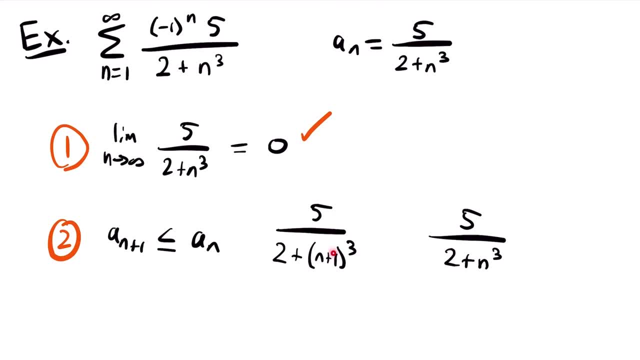 the value of this fraction will always be less than this fraction, And so we can say that it is true that a sub n plus 1 is less than or equal to a sub n, And so our second requirement is met, which means that our alternating series converges. 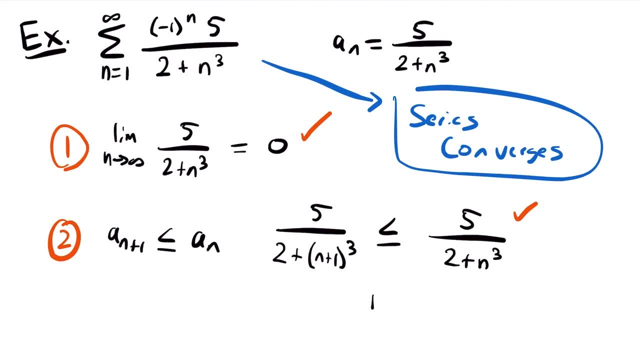 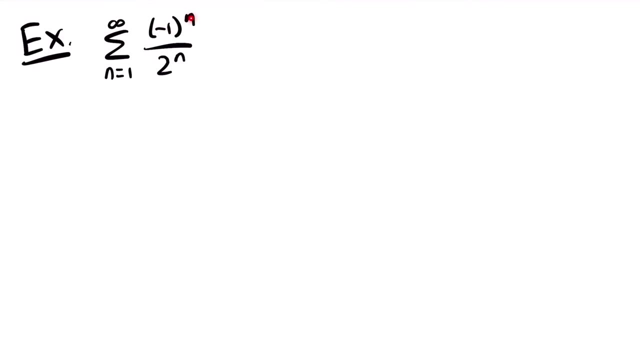 Okay. so since our series is decreasing for all values of n greater than or equal to 1, and the limit as n approaches infinity of the sequence is equal to 0, we know for a fact that this series converges. Here's another example. We have the sum from n equals 1 to infinity, of negative 1 to the power of n, divided by 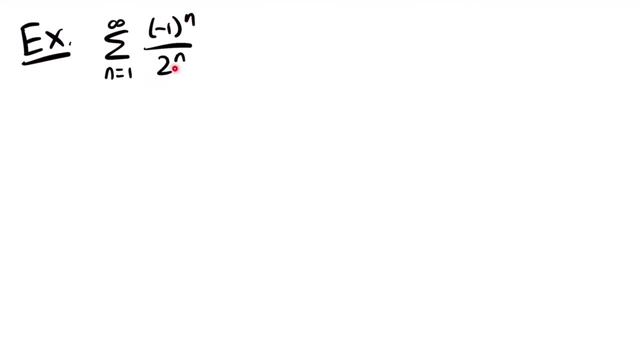 2 to the power of n, and once again, we can quickly identify this series as an alternating series because we have negative 1 to the power of n, and so we know that we can use the alternating series test to determine if this series converges or diverges. and so the first step is to find 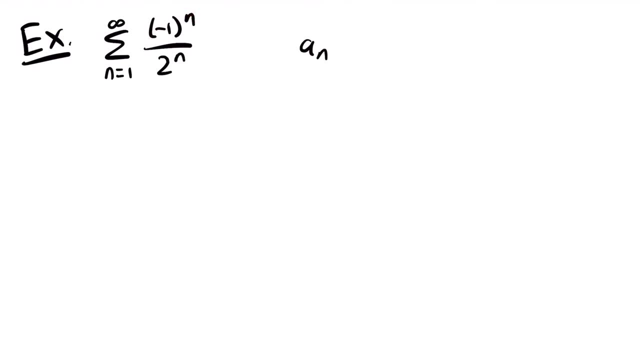 a sub n, and so in this case, if we block out negative 1 to the power of n, all we'll be left with is 1 divided by 2 to the power of n. Alright, so that is our sequence that we are going to be using for our test. 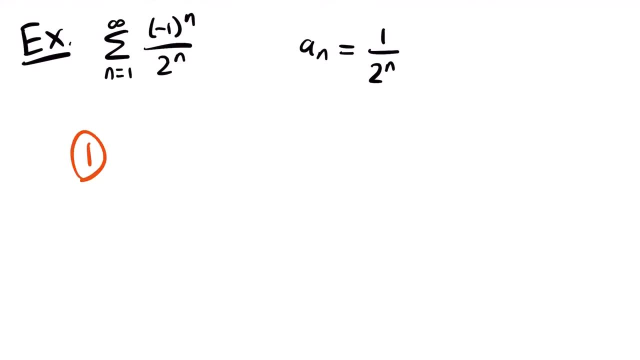 Okay, and so let's check our first requirement for the alternating series test. Let's take the limit: as n approaches infinity of 1, divided by 2 to the power of n. and as n approaches infinity, 2 to the power of n is going to continually increase. 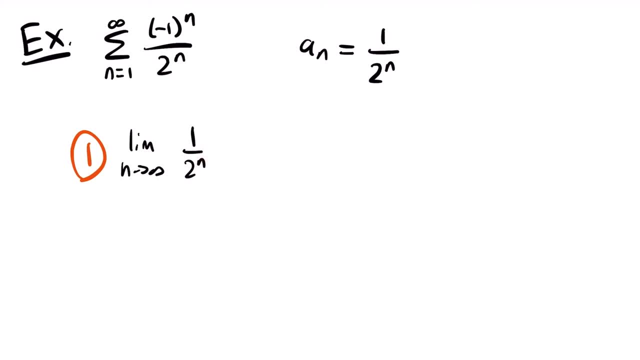 2 is being raised to a higher and higher power, and so it's getting larger and larger. So we have a fixed value of 1 divided by an increasing denominator, which will approach 0 as n approaches infinity. Alright, so the first requirement is met. 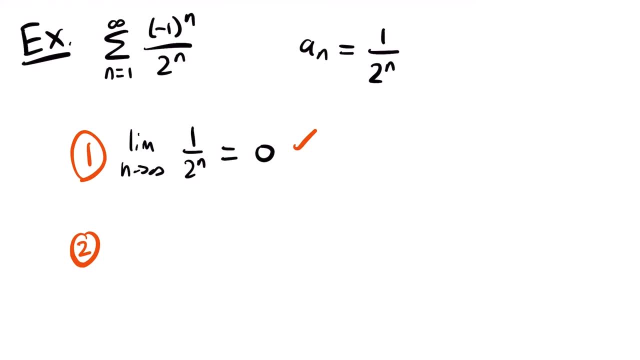 Now let's check the second one. Let's see if our sequence is a decreasing sequence. So we need to show that a sub n plus 1 is less than or equal to a sub n, and in this case a sub n plus 1 will be 1 divided by 2 to the power of n plus 1, and we are comparing. 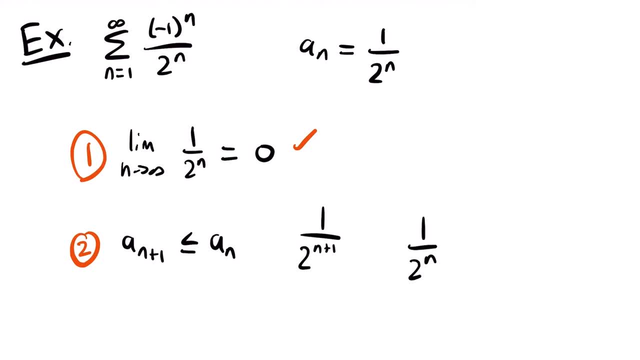 that to 1 divided by 2 to the power of n. Alright, now if we compare these two fractions, the denominators are what differ, and so 2 to the power of n plus 1.. 1 is always going to be greater than 2 to the power of n. 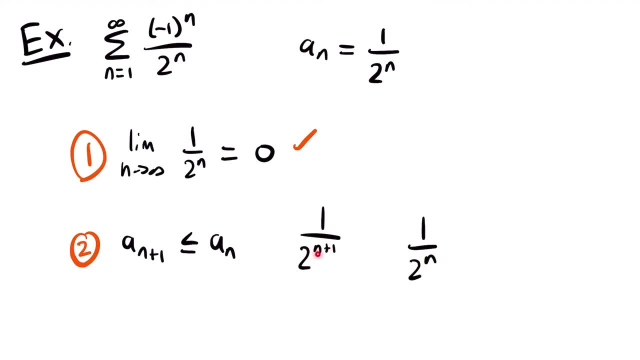 Right, for whatever value of n we are using, this power is always going to be 1 greater than this power. It's n plus 1, and so this denominator will be greater than this denominator, and so, since that denominator is greater, this fraction will be less than this fraction, and so for. 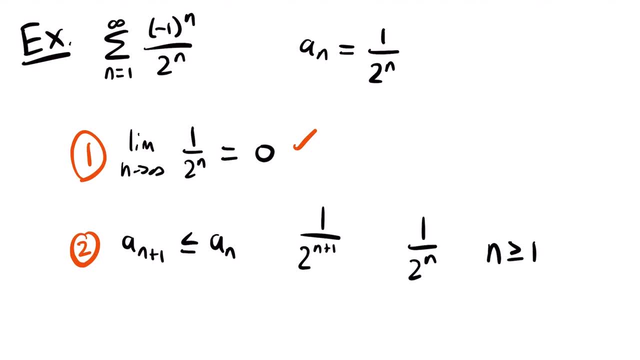 all values of n greater than or equal to 1, this fraction, or a sub n plus 1, will be less than or equal. That's where we are going to work on the general equation of n. So negative 1 to the power of n is equal to 1 divided by 2 to the power of n. 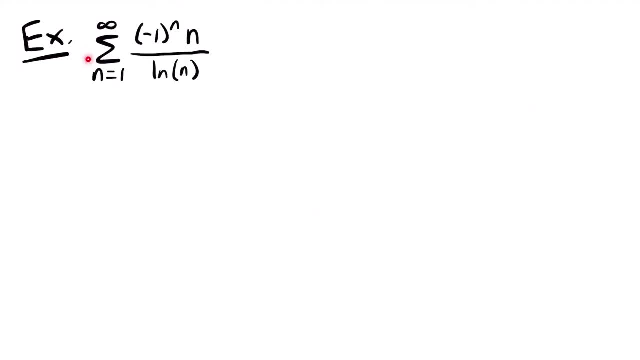 So our second requirement is met. We can now conclude that this alternating series converges. Okay, here's one more example for us to look at For this series. we have the sum from n equals 1 to infinity of negative, 1 to the power of. 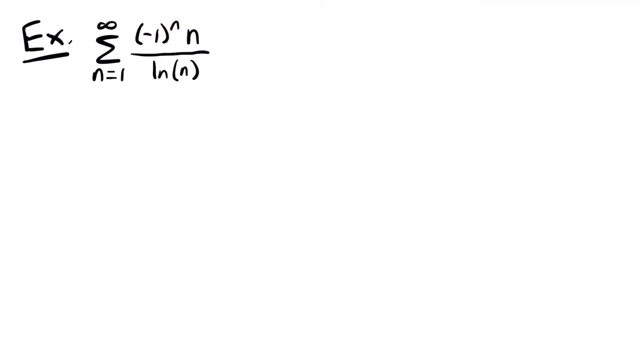 n times n, divided by the natural log of n. Alright, so we know that this series is an alternating series, And so we know that we can use the alternating series test to determine whether it converges or diverges. And so let's identify. 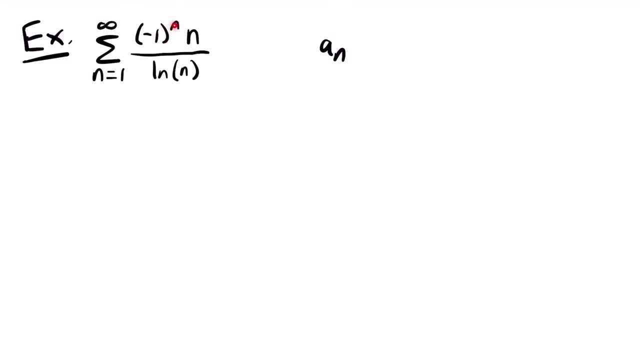 our sequence, a sub n. If we remove negative 1 to the power of n, what we will be left with is n divided by the natural log of n. Alright, and so if we look at our first requirement, let's check the limit as n approaches infinity, of n divided by the natural log of n. And 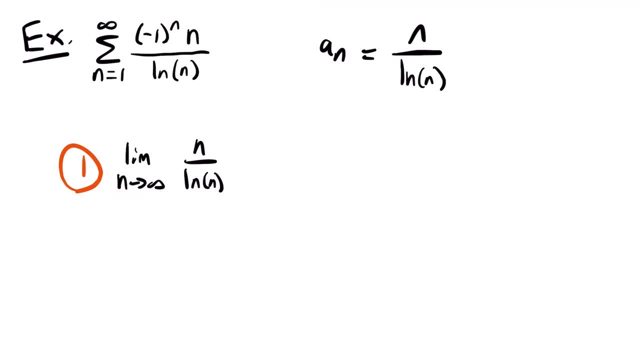 so what happens to this expression as n approaches infinity? Well, in the numerator n is approaching infinity, so we have infinity in the numerator, And then in the denominator we have the natural log of n, and n is approaching infinity, And so we are inputting larger and larger values. 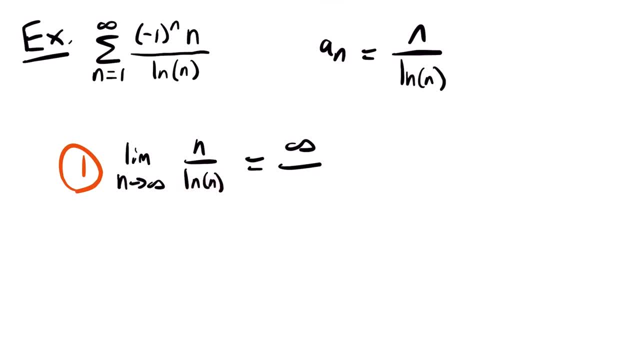 into the natural log function. And as you input larger values into the natural log function, it's going to output larger values, So the denominator is also increasing to infinity. So we have an indeterminate form For our limit, which means that we can use L'Hopital's rule to simplify it and then try. 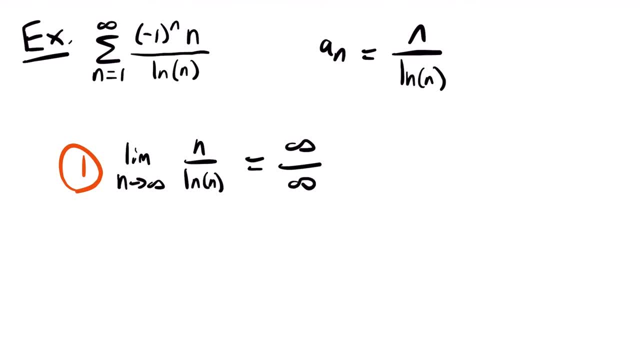 to evaluate again. So what we can do is take the derivative of the numerator and denominator with respect to n. Alright, so if we do that, this will be equal to the limit, as n approaches infinity, of the derivative of n, which is just going to be 1,. right, When you take the. 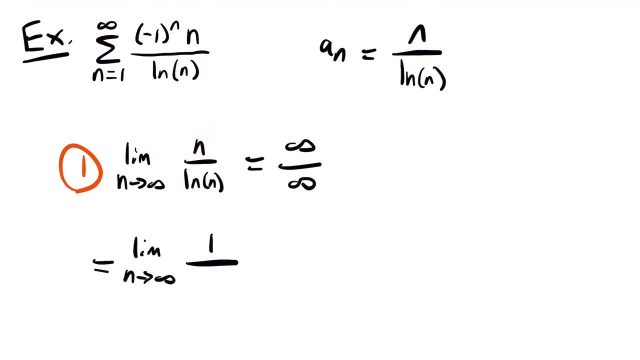 derivative of a variable to the power of 1, it's just equal to the coefficient, which is 1. in this case, The denominator will take the derivative of the natural log of n, and the derivative of the natural log of n is just 1 divided by n. okay, So now if we simplify 1 divided, 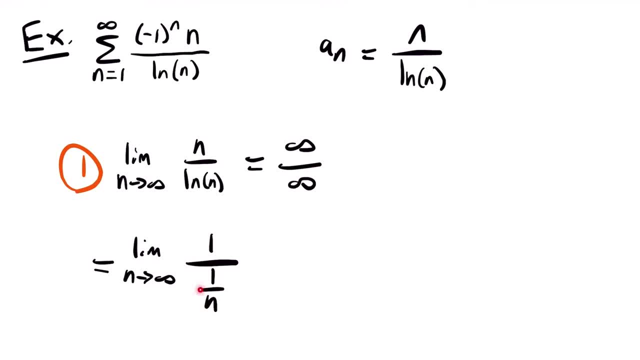 by 1 divided by n will be the reciprocal of 1 divided by n, and so this is equal to the limit, as n approaches infinity, of n divided by 1, but that's just equal to n, and so I'll rewrite that to be n, And as n approaches infinity, this n approaches infinity, So we're. 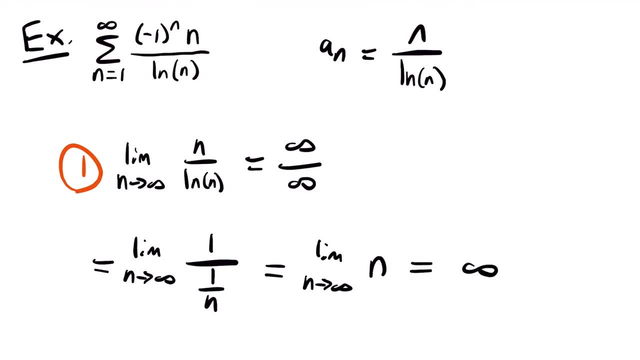 going to have. n approaches infinity, And so this limit is equal to infinity, which is not equal to 0. And so our first requirement for the alternating series test is not met. In fact, we have shown via the divergence test, by taking the limit of our sequence, that 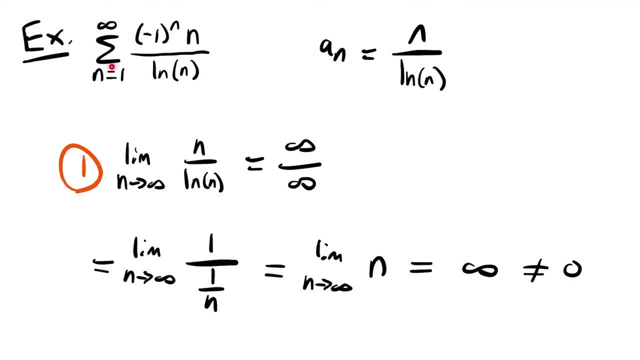 that limit is not equal to 0,, which means that this series diverges Alright, and so that is the final answer for this example: This alternating series diverges Alright. so we're going to switch gears a little bit here. We're going to be looking. 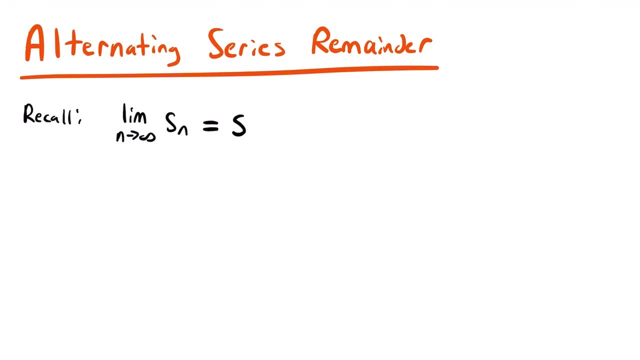 at how to approximate the sum of a convergent alternating series. Alright, so, unlike some of our other special types of series, such as a geometric series, we're not going to be able to calculate the sum of an alternating series using a nice formula. However, we are. 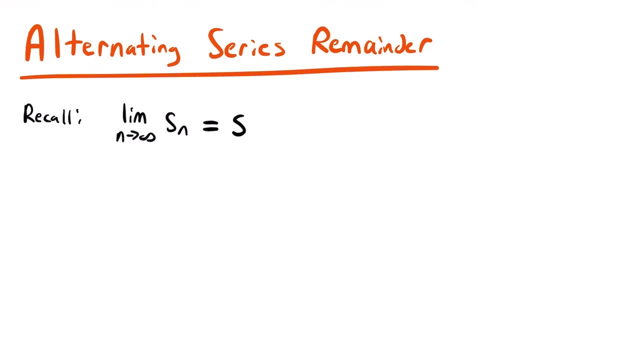 able to approximate the sum of an alternating series because of how the terms are decreasing and alternating, And so we'll talk about that in a little bit. but first I want you to recall that when we first looked at series, we said that we could find the sum of the series or the value that 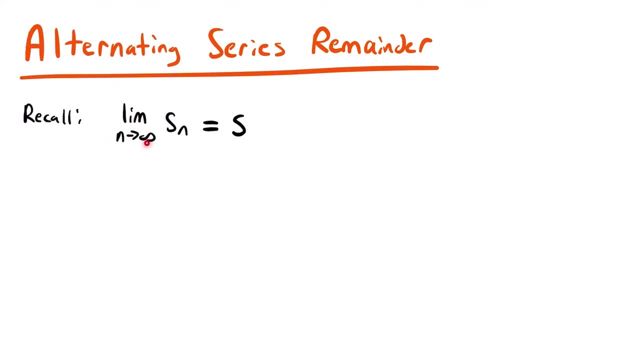 it converges to, by taking the limit as n approaches infinity of the nth partial sum, And if that limit exists, then that would be the sum of the series. Alright, and so if that is true, then we could also say that the limit as n approaches infinity of the sum of the series. 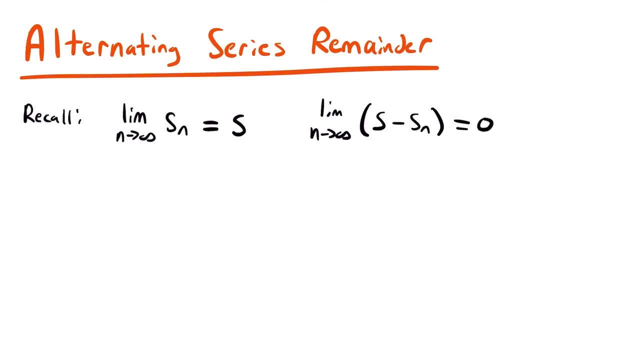 minus S sub n would be equal to zero, Right? so if the limit as n approaches infinity of S sub n is equal to S, then the limit as n approaches infinity of the sum of the series minus S sub n should be equal to zero. Alright, and so that would be true for n approaching. 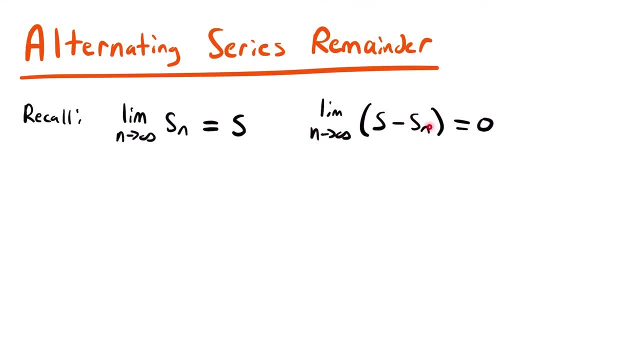 infinity. but if we don't look at all values of n for our partial sums, there's going to be a measurable difference between the actual sum of the series and whatever partial sum we're looking at. Alright, and so this is kind of what we're trying to figure out, and 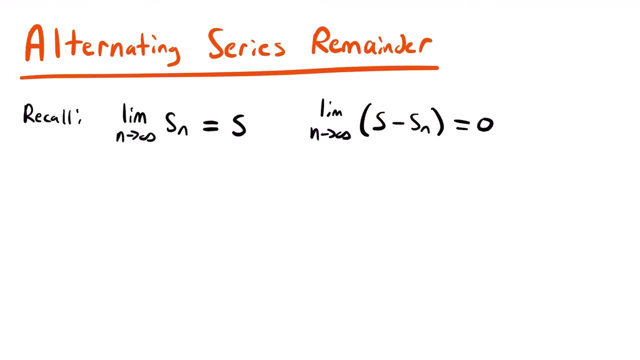 where the idea of approximating the sum of an alternating series comes from. And so what we're going to say is that the sum of the alternating series is approximately equal to some partial sum- S sub n- And because that partial sum is approximately equal to the sum of the series, there's going. 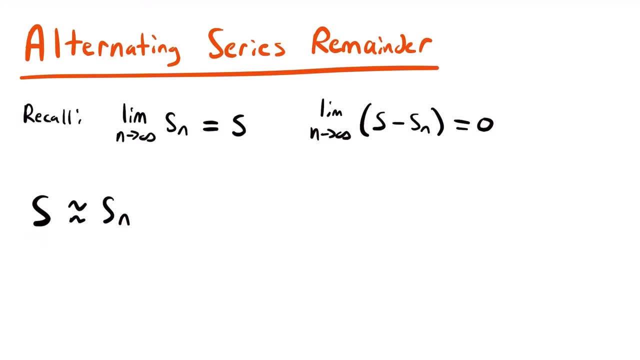 to be a difference between those values that we can measure And we call that difference the error or the remainder for the sum And we're going to label that with capital R sub n. So the error or the remainder will be equal to the difference between the actual sum of 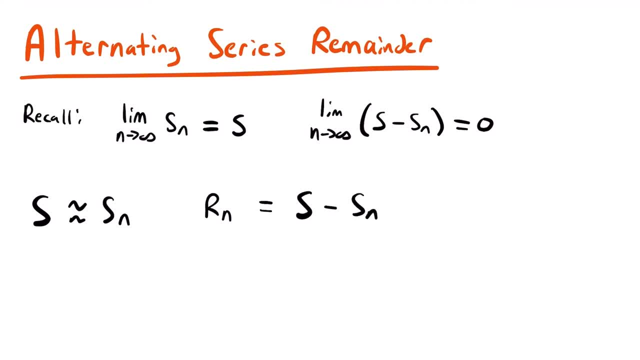 the series and the nth partial sum right. Another way you could look at that is that the error is equal to the whole sum minus part of the sum. all right, And so what we can do is calculate a partial sum that is approximately equal to the whole. 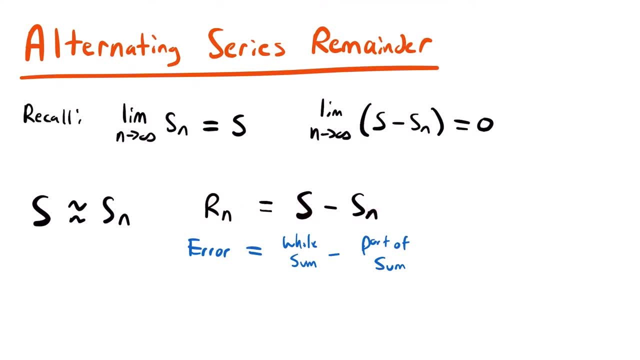 sum Within some margin of error, okay, And so we don't actually care about the sign of that error or the difference between the whole sum and part of the sum, And so it could be negative or positive, we don't care. And so we're actually going to look at the absolute value of the error, or the absolute 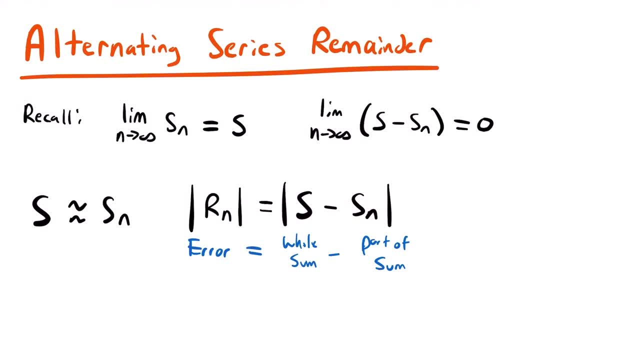 value of the difference between the whole sum and part of the sum. And what we know about this error for an alternating series that converges is that that error will be less than or equal to a sub n plus 1,. all right, Now it seems like that kind of came out of nowhere, but here's why that is true. 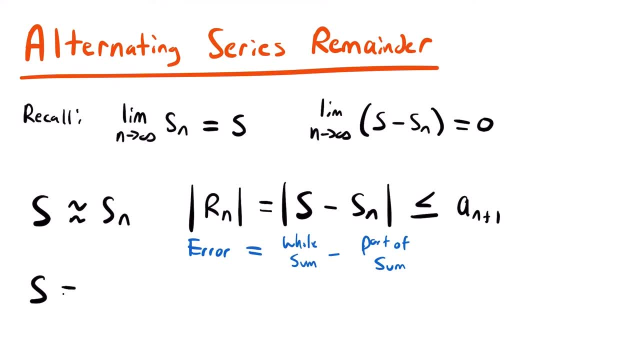 If we look at the sum of an alternating series, that would be equal to the first term, a sub 1- and then the next term would need to be negative, right? So we'd have minus a sub 2, then plus a sub 3, and that could continue on for a while. 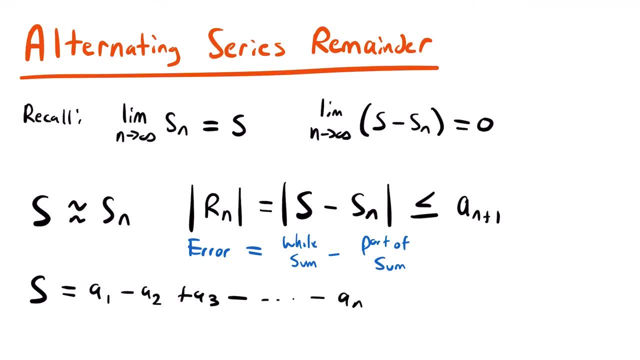 So we'll subtract the next term and then we'll move on to a sub n and then add a sub n plus plus 1,, subtract a sub n plus 2, and so on. right, We're adding up all of the terms of the alternating series. 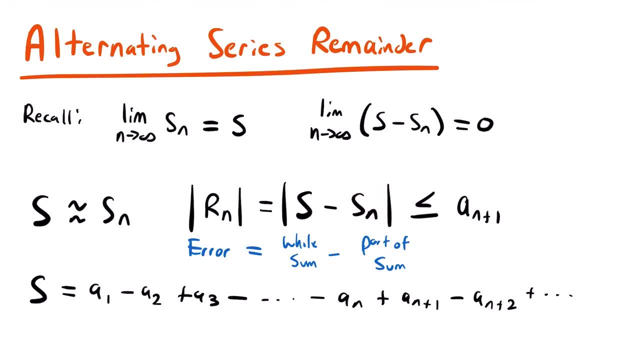 If we calculate a partial sum s sub n, that is going to add up all the terms of our alternating series up until a sub n, right? So all of these terms right here represent the nth partial sum, And then what's left over is the difference between the actual sum of the 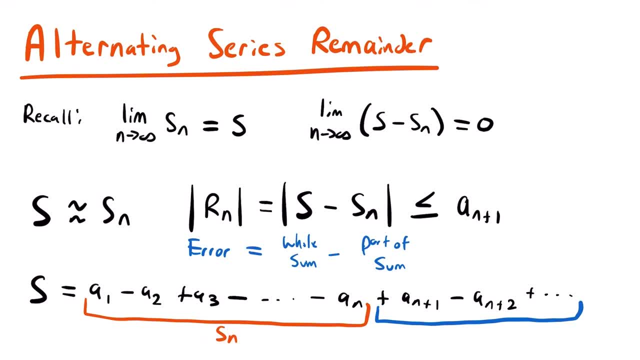 alternating series and our partial sum, right. So whatever this partial sum is that we calculated, the difference between that and the actual sum are the left over terms, And so we would say that these terms are s minus, s sub n, And so the reason why this difference is less than or equal to a sub n plus 1 is because 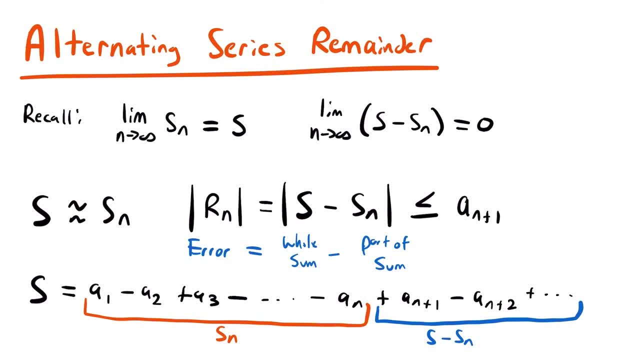 the terms of a converging alternating series are decreasing. right, since we are assuming that this is the sum of a convergent alternating series, Then our sequence, a sub n, needs to be decreasing, which means that the absolute value of each of our terms will be smaller than the previous term. 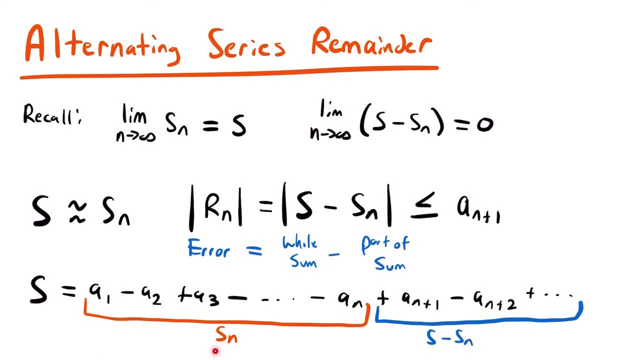 And so, because of that fact, after we stop calculating s sub n, the value of a sub n plus 1 is the largest that the difference between the partial sum and the actual sum could be. The rest of these terms, as we add them to our sum, will not take us back to the value. 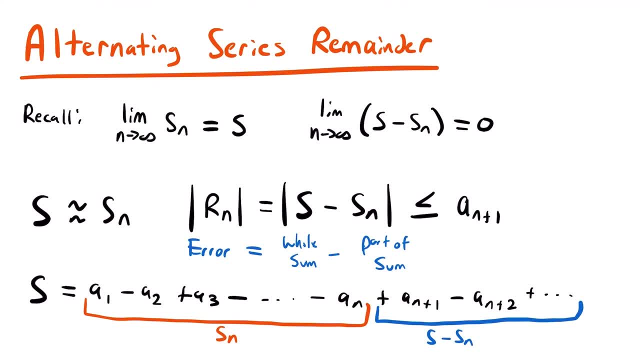 of a sub n plus 1, right. So, for example, Let's just say that a sub n plus 1 was equal to 10. The next term we would be subtracting would be smaller than 10.. Let's say that it is 9.. 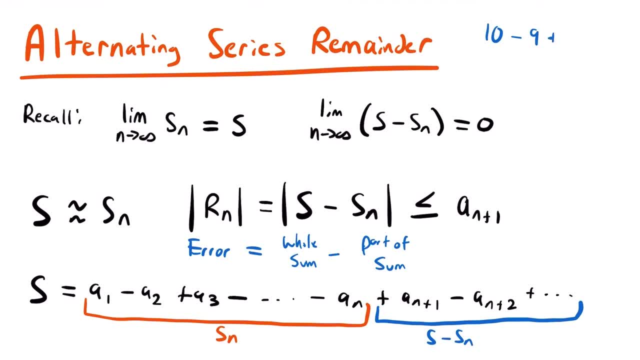 And then the next term would have a smaller value than 9.. So we would be adding, let's say, 8, and then subtracting 7, and then adding 6, and so on. If these were the terms of our series right here you can see that 10 is the largest value. 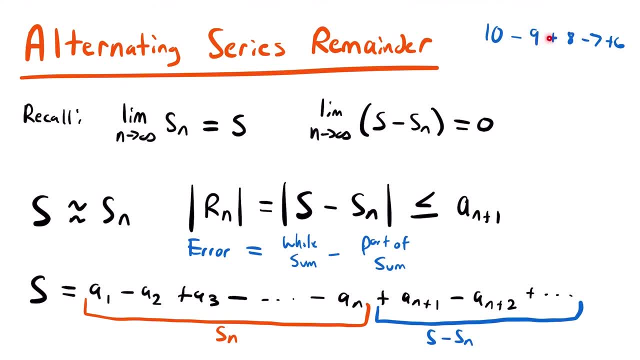 that these terms will be: 10 minus 9 is 1, plus 8 is 9.. That never got back to 10.. 9 minus 7 is 2, plus 6 is 8.. That also will never get back to 10.. 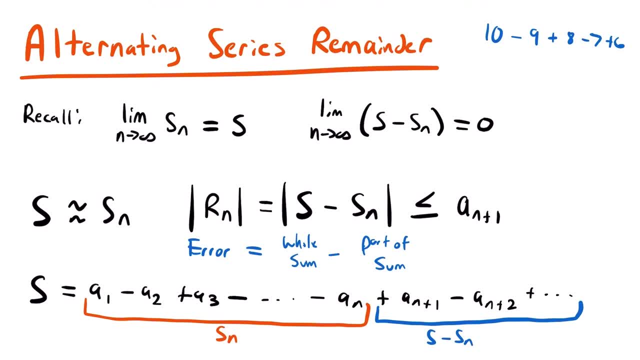 So, as we continue to add more and more of our terms, of the sequence, this first term, after we stopped calculating s sub n, which is a sub n plus 1, represents the value for which our error or the difference will be less than or equal to. 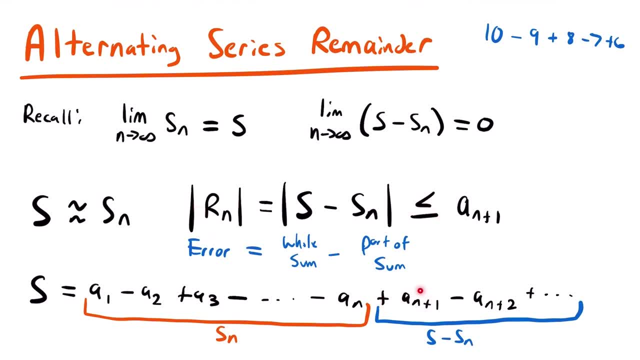 The error will not be larger than the value of that term. Okay, So hopefully that made sense. It's a little bit of a difficult concept to wrap your head around, so maybe you need to go back and rewatch that explanation again And if you have any questions, leave them in the comments. 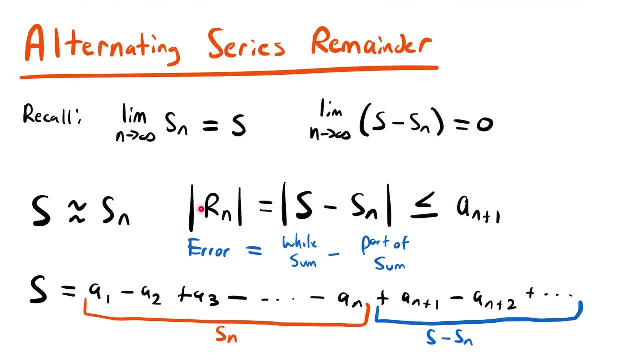 But the important takeaway here is this equation right here, that the error or the difference between a partial sum and the actual sum of our alternating series will be less than or equal to the n plus 1 term, a sub n plus 1.. 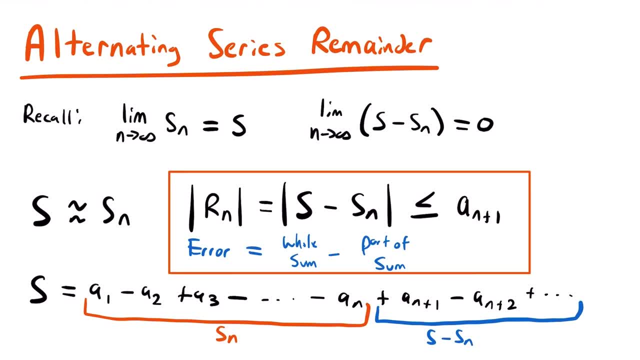 Alright, And so this is the formula that you want to have written down somewhere, Because that's what you are going to use when you approximate the sum of an alternating series, And what we're going to be able to do with this formula is tell it how close to the actual 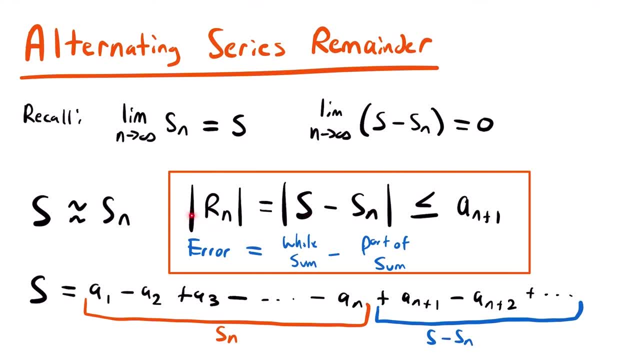 sum of the alternating series. do we want to be, and use that value to determine how many terms n we need to be that accurate, Alright. And so to make sense of what I mean by that, let's take a look at an example where we will. 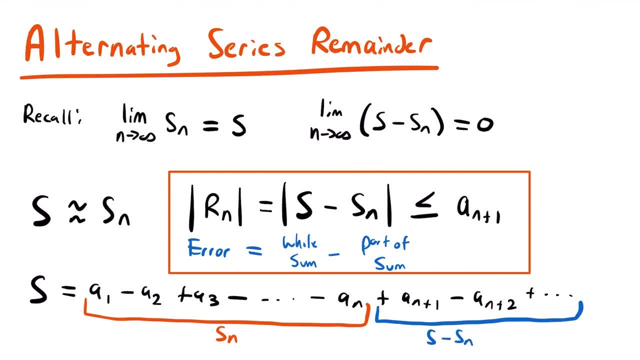 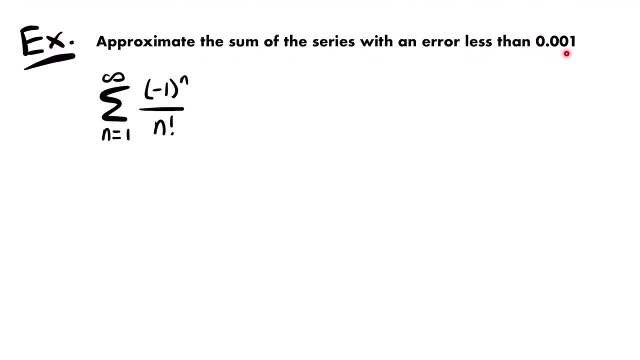 approximate the sum of an alternating series. Okay, Alright. so here's our example. We want to approximate the sum of the series with an error less than 0.001.. Alright, so this value right here is telling us how close we want our approximation of. 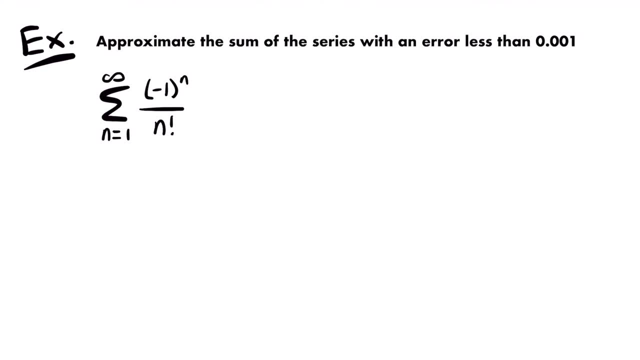 the sum to be, We want our approximation to be accurate for at least the first two decimal places. Okay, so now, before we do anything with the error formula, before we try to approximate any sums, we first need to check that this alternating series does connect. 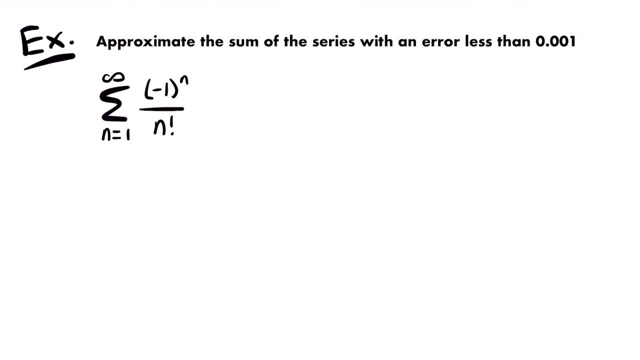 Okay, And so let's use the alternating series test. In this case, a sub n is going to be equal to 1 divided by n. factorial Right. We just removed negative 1 to the power of n to get our sequence, And so let's check the first requirement. 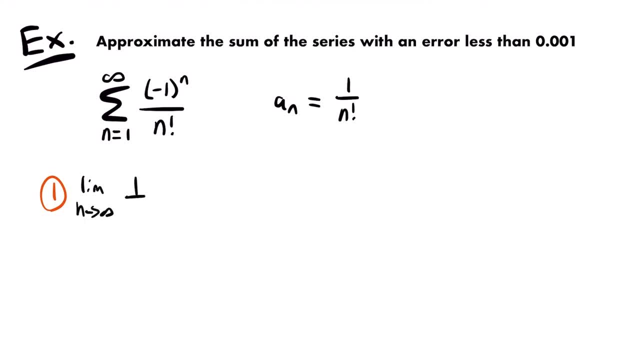 Let's take a look at the limit, as n approaches infinity, of 1 divided by n factorial. Alright, and so what happens to 1 divided by n factorial as n approaches infinity? Well, as this value of n gets larger, the value of the factor n is going to be 1 divided. 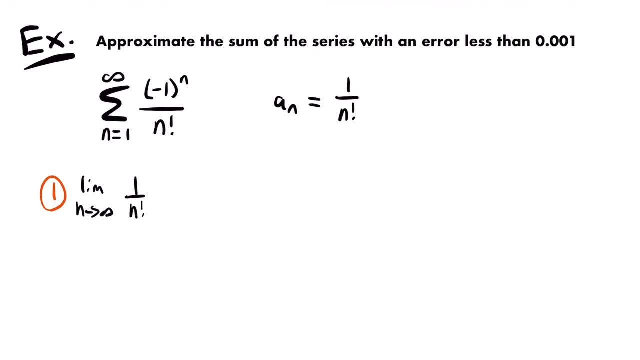 by n factorial, And so we know that the factorial is going to get larger. Right? 2 factorial is equal to 1 times 2,, 3 factorial is equal to 1 times 2 times 3, and 4 factorial is equal to 1 times 2 times 3 times 4.. 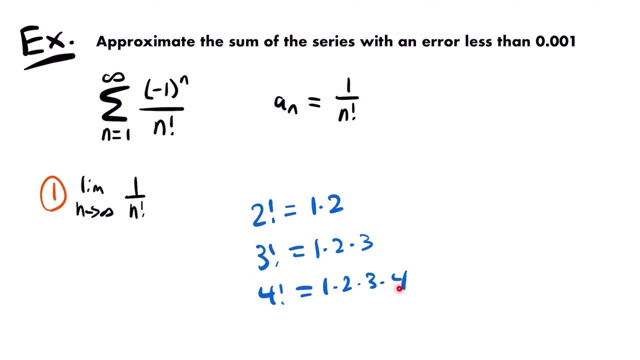 So as the value of n for the factorial increases, so does the value of that denominator, And so we have a fixed value divided by an increasing denominator, and so we know that this limit will be equal to 0.. Alright, 1 divided by n- factorial. 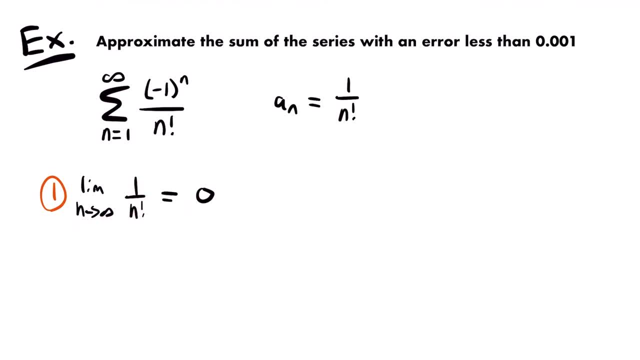 Alright, n approaches infinity, will approach 0.. Okay, And so our first requirement is met. Now we need to check the second requirement that a sub n plus 1 is less than or equal to a sub n. And so now, if we look at a sub n plus 1, that will be 1 divided by n plus 1 factorial. and. 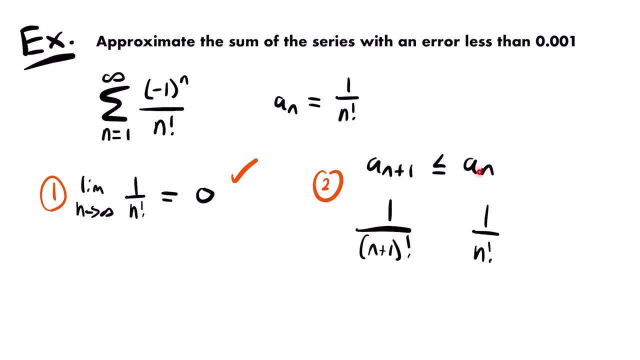 we're comparing that to 1 divided by n factorial, That is a sub n. Okay, And so can we conclude that this term will always be less than or equal to the value of a sub n. Well, if you look at the denominators, this denominator is always going to be greater. 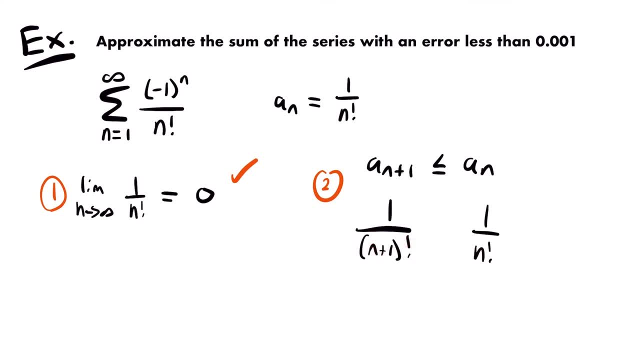 than this denominator. because we have n plus 1- factorial, This denominator will always be a larger value, And so, since that denominator will be larger, the value of this fraction will be smaller than this fraction, And so we know that a sub n plus 1 will be less than or equal to a sub n. 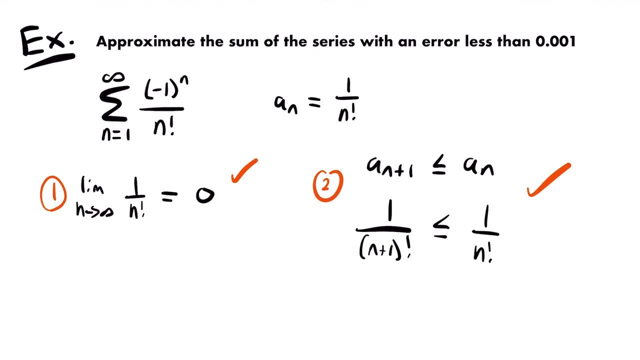 And so that checks out. We now know- We know via the alternating series test- that this alternating series converges. Okay, So that's what we needed to check. You always need to check that first before you approximate the sum of an alternating series. 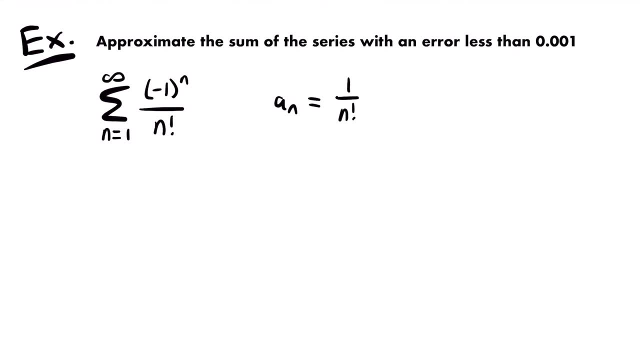 You need to be sure that it converges. Alright, but now to approximate the sum, we're going to be using this formula: that the absolute value of the error is equal to the absolute value of the sum minus the nth partial sum, and that is less than or equal to a sub n plus 1.. 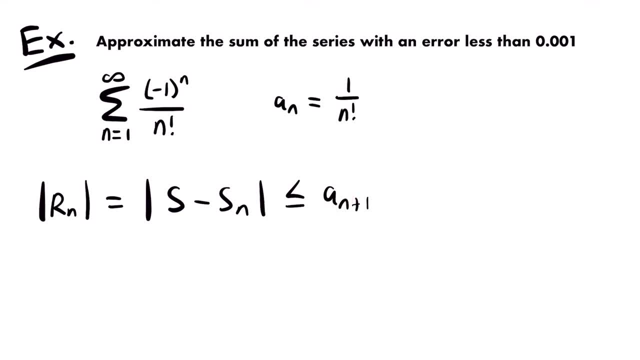 Okay, And so what is a sub n plus 1 for our sequence? Well, that's going to be equal to 1 divided by n plus 1, factorial Right. We just replace n with n plus 1, and that is the term: a sub n plus 1.. 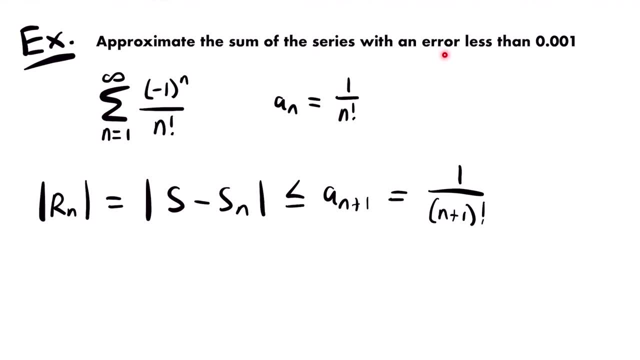 Alright, now for this approximation. we know we want the error to be less than 0.001.. And so the difference between the sum of the series and the nth partial sum which is less than or equal to the term- a sub n plus 1, needs to be equal to 0.001. 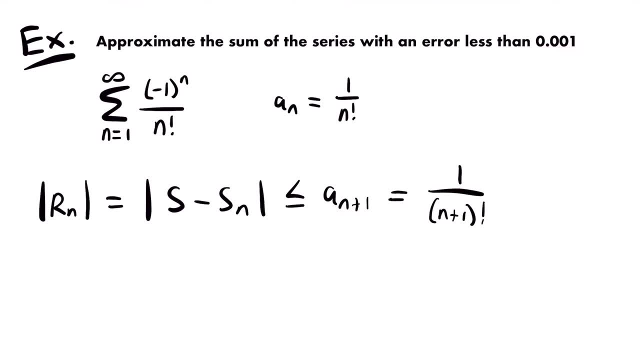 Okay, So we would say that the error r sub n is less than or equal to a sub n plus 1, which is 1 divided by n plus 1, factorial, and we want that to be less than 0.001.. 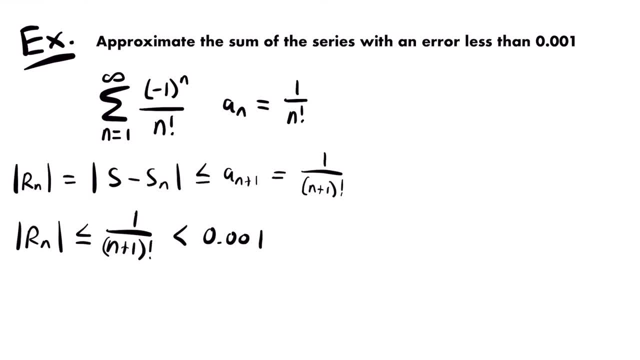 Okay, And so now, if I clean up my work a little bit, what we want to do is determine what value of n will make this inequality true Right. When will 1 divided by n plus 1 factorial equal to 0.001?? 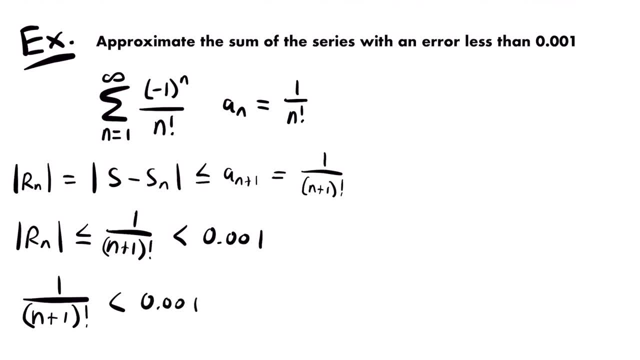 Right? Well, if we manipulate this a little bit, if we take the reciprocal of both sides, meaning we flip the numerator and denominator, that will also flip this inequality. so it will change from being less than to greater than, and so if we do that, it will look like this: 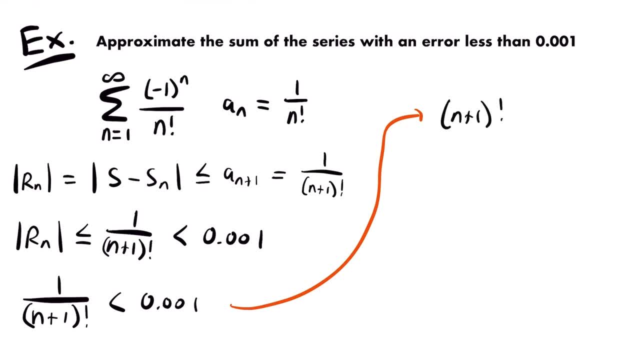 We'll have n plus 1 factorial is greater than 1 divided by 0.001.. Right, So we just took the reciprocal of both sides of the inequality and then flipped the inequality to be greater than Alright. And now 1 divided by 0.001 is 1,000, and so I'm just going to rewrite that to be 1,000.. 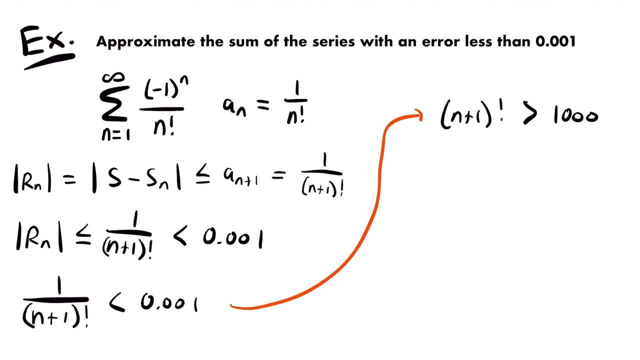 Okay, And so now all we have to do is ask ourselves what value of n plus 1 factorial is greater than 1,000?. Alright, now for some series. it's going to be a lot easier to solve for n, but in this, 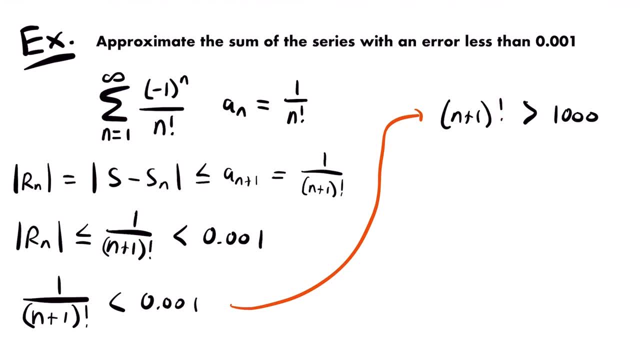 case, we have to do a little bit of guessing. because of this factorial, It's not as easy to solve for n, Right? So let's try some values. If n is equal to 5, then we have 5 plus 1 factorial, which is equal to 6 factorial. 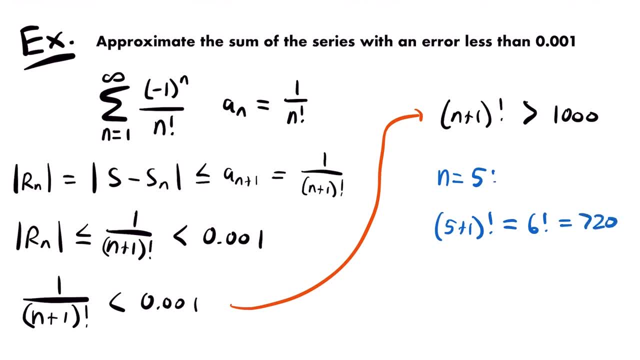 and 6 factorial is equal to 720,, so that is less than 1,000.. So now let's try: n is equal to 6, so we'd have 6 plus 1 factorial, and that will be equal to 7 factorial, which is equal to 5,040, and so that's way bigger than 1,000, and so 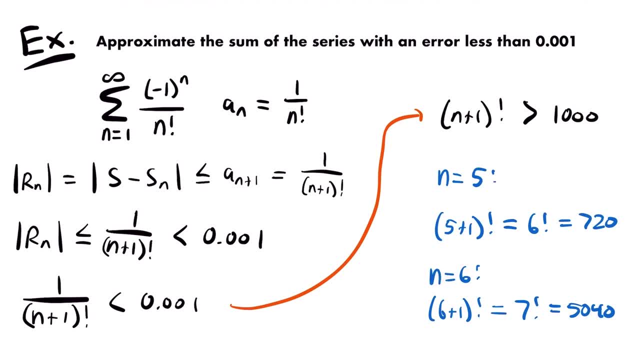 that's the value of n That's going to make this statement true. Alright, so what we have found is that when n equals 6, the error for our nth partial sum compared to the actual sum of the series will be less than 0.001.. 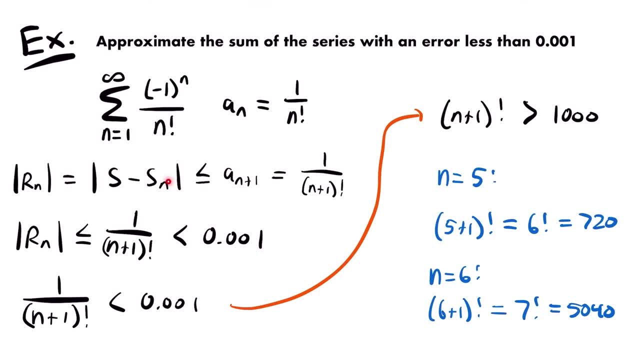 Alright. so if we calculate the partial sum, where n is equal to 6, we will have approximated the sum of the series with an error less than 0.001.. Okay, So n equals 6 is the value we are going to use. 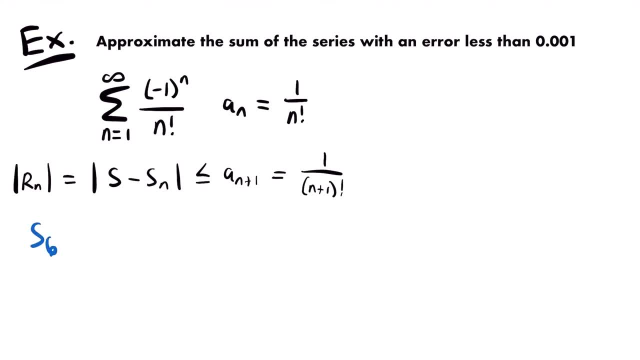 So, if I clean up my work here, Let's calculate s sub 6.. The sixth partial sum is going to be our approximation for the sum of this alternating series. that will have an error less than 0.001.. Alright, now the first term of our series, when n equals 1, will be negative 1 to the. 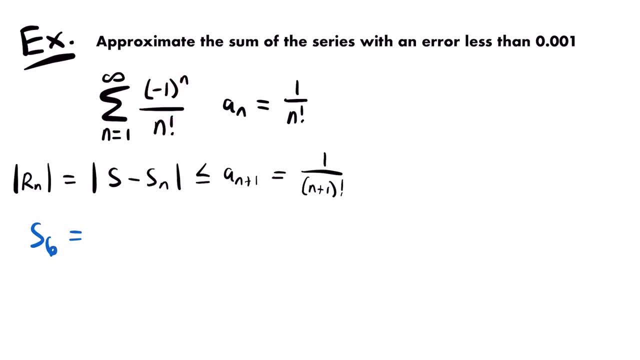 first power, which is negative 1 divided by 1 factorial. so we have negative 1 divided by 1 factorial, then our next term will be positive, because this is an alternating series. and then we'll have 1 divided by 2 factorial when n is equal to 2, then we will subtract. 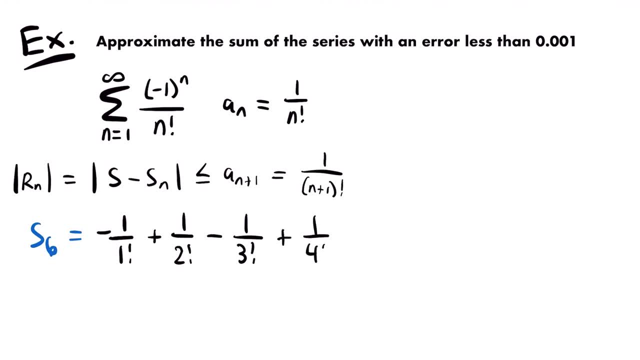 1 divided by 3 factorial, then add 1 divided by 4 factorial, subtract 1 divided by 5 factorial and add 1 divided by 6 factorial, And so those are the first six terms of our series. And so now, if we simplify these terms and add them together, it'll look like this: 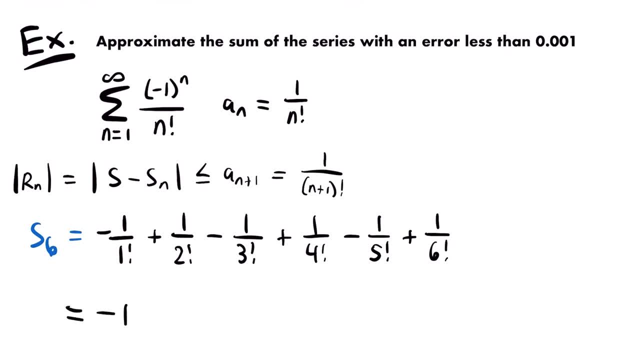 This is equal to negative 1, because 1 factorial is 1.. So negative 1 divided by 1 is negative 1, plus 1 half, because 2 factorial is 2.. Then 3 factorial is 6, so we have minus 1 sixth, plus 1 divided by 4 factorial, which. 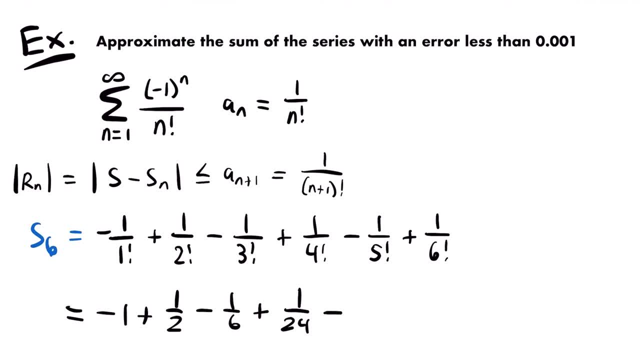 is 24, so 1 divided by 24, minus 1 divided by 5 factorial, which is 120,, plus 1 divided by 6 factorial, which is 720.. And so if you add all these terms together in a calculator, you will find that s sub. 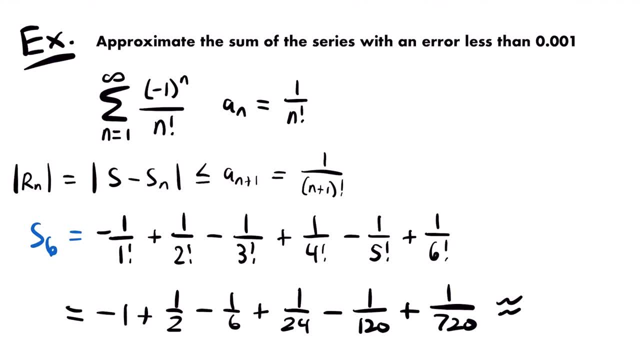 6, or the sixth partial sum is approximately equal to negative 0.63194, and some more decimals, And so that is the approximation of the sum of this alternating series, with an error less than 0.001.. All right, and so that is how you can approximate the sum of a convergent alternating series.